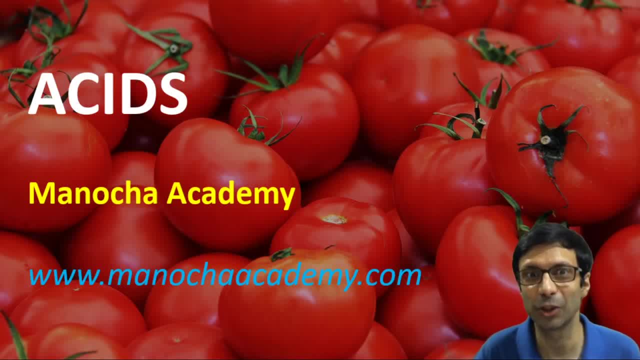 Hi friends welcome to this class on the acid based salt chapter and in this video we'll be focused on the acids part and I'm going to make the concepts really easy for you so I'm sure you'll really understand what acids are. I'm going to show you the tips and tricks on how to write the reactions and how to predict the reactions for the acids so you'll find the topic really easy. 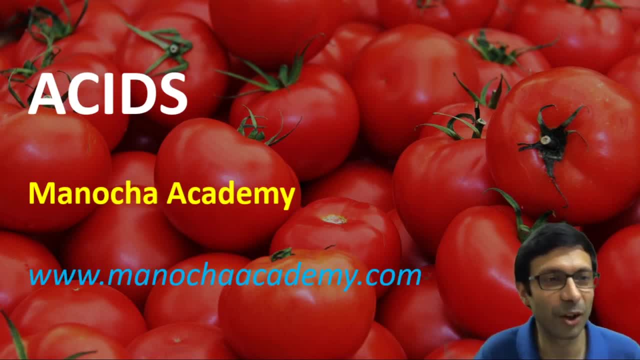 So hi I see a lot of folks are here on the chat so thanks for joining in on this live session on the acids topic. So I see Madhu is here, Vinita hi, hi Srinivas, hi Yash Gaming, hi Gamer Galaxy, hi Arjun Singh, hi Arun Ahmed, hi Rahul Dutt. So sorry if I can't take everybody's names. Hi showman Mukherjee, hi Gautam Devnath. So welcome to this class on the acids base bases and salts chapter and we are going to be focusing on acids. 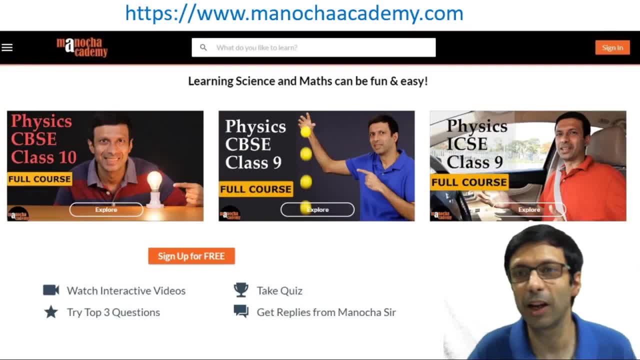 And guys you can check out my website manuchacademy.com. So we have courses here and we are excited to let you know that we've also launched the ICSE class 9 course so if you're on the ICSE board do check out the physics course for class 9. So we have these different courses 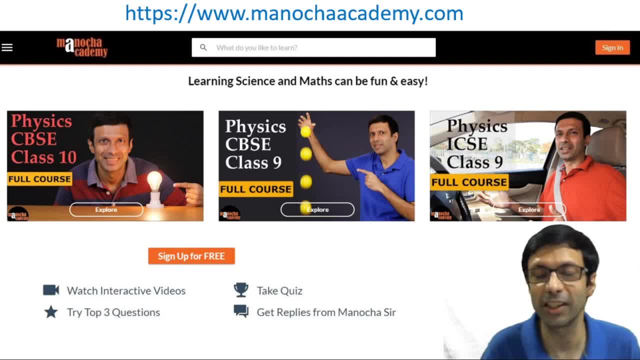 on the website for you to check out and they have videos, quizzes and questions and I'm sure you'll find them really useful. So hi Venu, hi Upendra Singh, hi Guru Darshan. 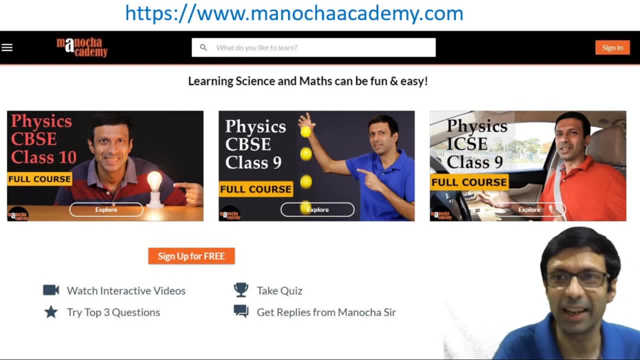 Hi Maya, so good evening welcome to this class and let's get started with the acids topic. So I'm going to make the concepts really easy and be sure to watch the entire class I'm sure you'll enjoy it. 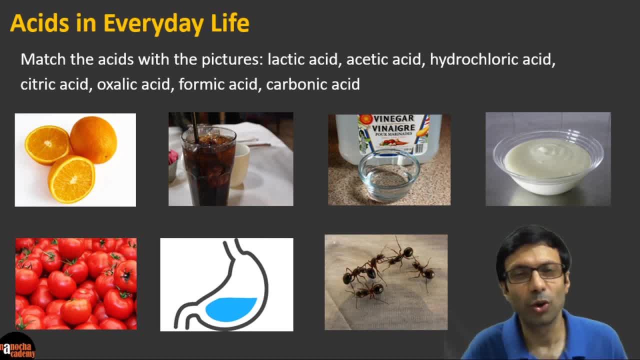 So let's start with acids in everyday life. So you must be familiar that we are using or we come across acids in our daily lives. So I have an interesting question here for you where you need to match the pictures with the acid list that is given here. So can you see that there's a list of acids given right here okay and you need to match the pictures with the acids and 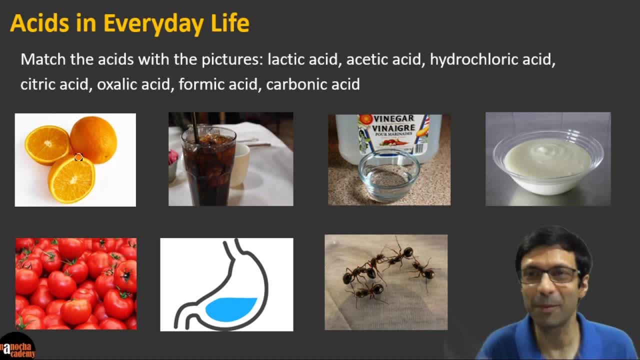 guys if you haven't hit the like button do hit it like right now and also subscribe to our YouTube channel Manochacademy.com and click on the notification bell so that you get notified about the new videos. Alright guys so let's go ahead and start with this one. So let's start 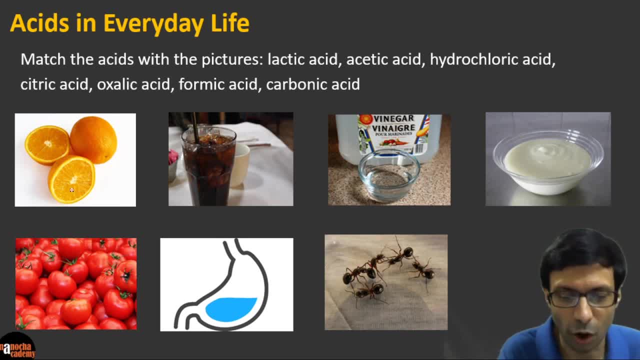 okay so which acid is present in the orange so let's go picture by picture I 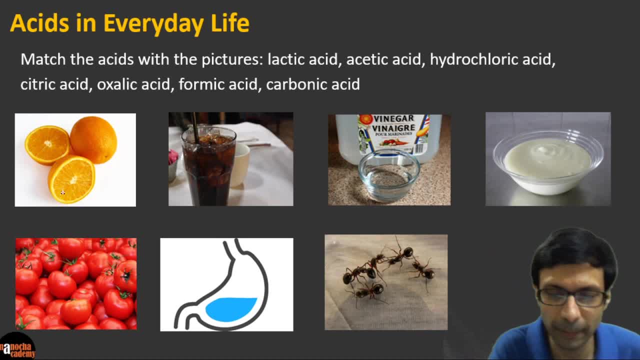 can see a lot of good answers coming on the chat so let's go one by one so let's start with the orange right here okay can you see that so what acid is present 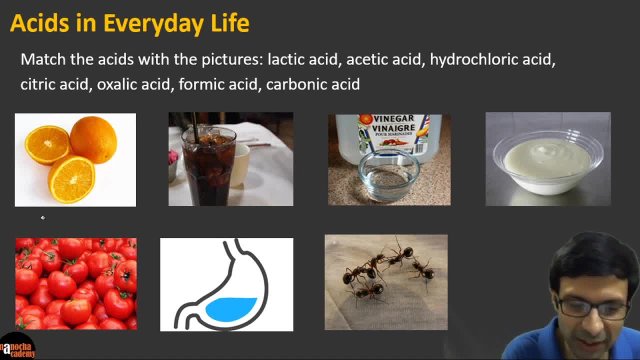 in the orange excellent I see the right answer on the chat so you guys got it the main acid is citric acid right and you know orange contains vitamin C which 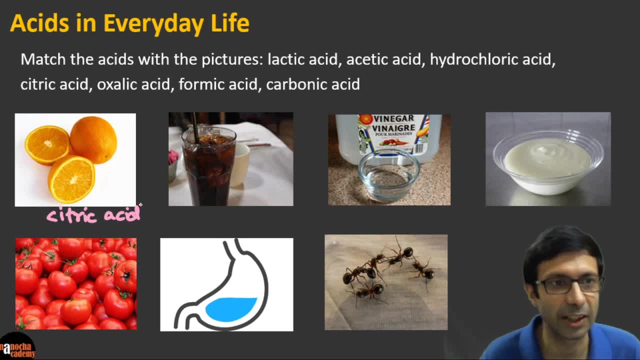 is as ascorbic acid but we are matching the ones on the list here excellent now 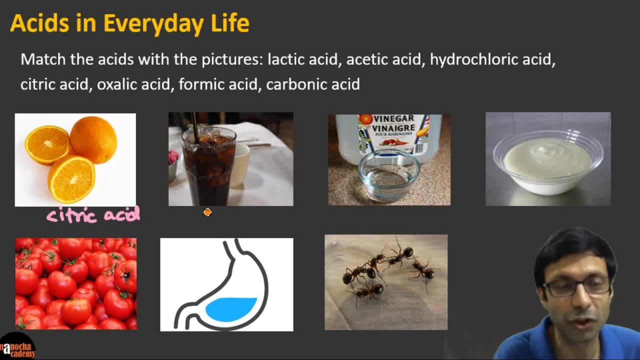 let's go on to the next picture so can you see this picture of a soda right so soda drink here so can you tell me what is the acid present in soda okay so from 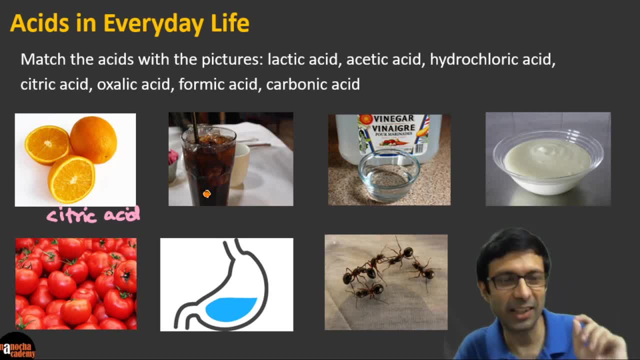 this list here what is the acid present super you guys are great you've got this one too so the acid is carbonic acid- xрыnt transferred so when you are 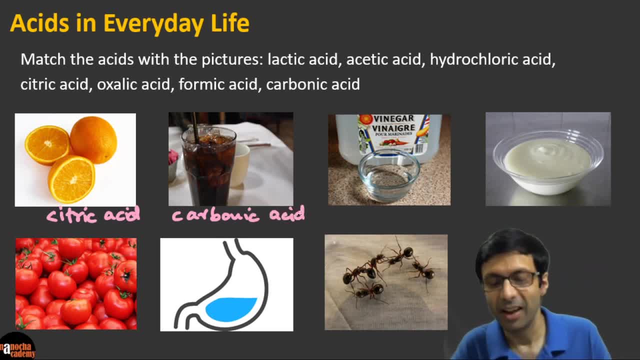 drinking a soda you're how toется actually consuming carbonic acid. Next, let's move on to the next picture here. Can you see the 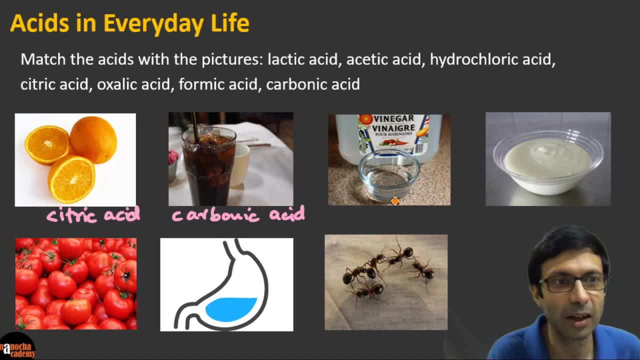 picture shows a bowl of vinegar, right? They poured vinegar from here. And what is the acid present in vinegar? So guys, can you tell me this one? Okay, excellent. I see the right answer. It's 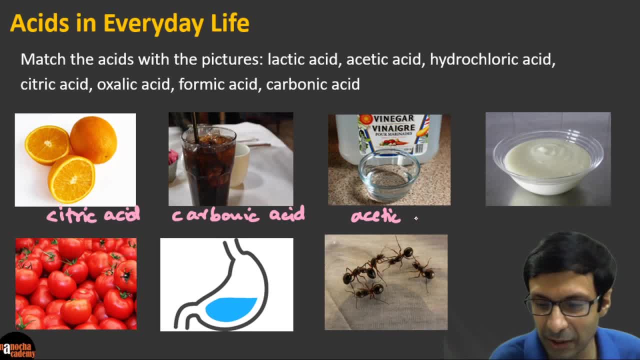 acetic acid. Okay, so that's the correct answer. So let's go ahead and take the ones that we've used. So we've used acetic acid here. We've used citric acid and carbonic acid was present in the cola drinks, right? Now let's go ahead to the next one. Can you see this bowl of curd or what we call 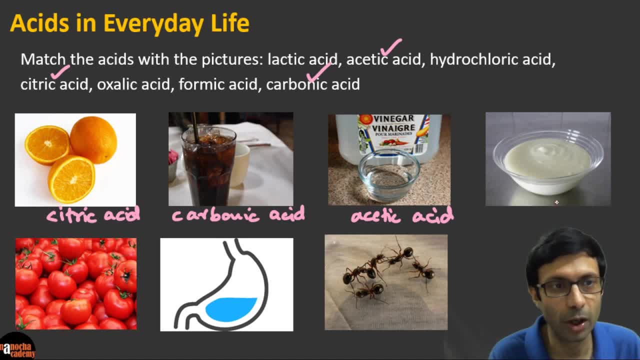 yogurt, right? So in this bowl of curd or yogurt, what is the acid present? Super, that's the right answer. The correct answer is lactic acid. Okay, so absolutely right. And let's take that one too. 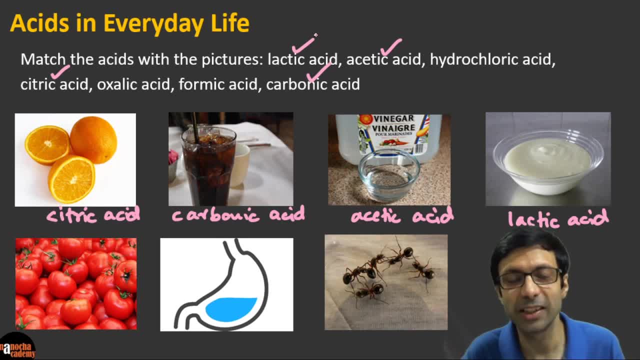 Now next, what is the acid present in tomatoes? So who can answer this one for me? So what is the acid present in tomatoes? Okay, so I see a lot of you are writing the correct answer, oxalic acid. Absolutely right. So tomatoes also contain citric acid, but it also contains oxalic acid. So we are trying to choose a unique one from the list since we've already used citric acid. So oxalic acid is 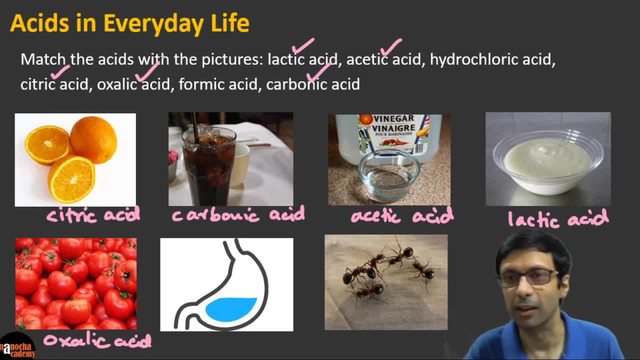 perfect answer. Next is the picture of a stomach here. And as you know, our stomach produces acid and that acid helps in the digestion of food. Okay, so guys, and I see some of you have written malic acid. That's also true. Tomatoes do contain an amount of malic acid also, but we are choosing 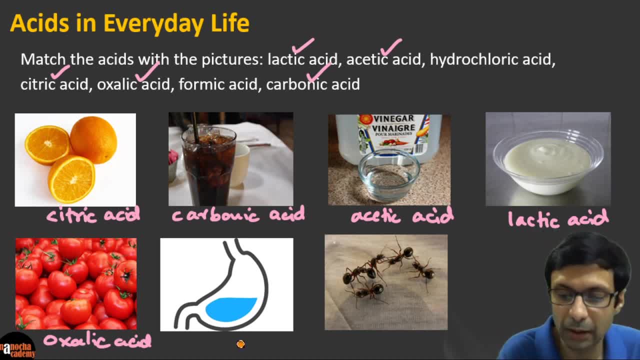 from the list given here, right? So guys, what is the main acid present in the stomach? Excellent. 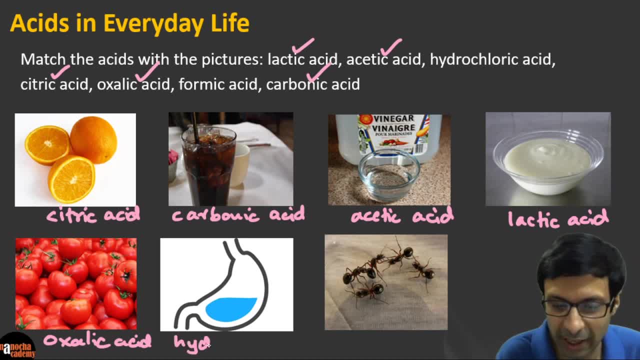 I see the correct answer. So the answer is hydrochloric acid. Perfect. 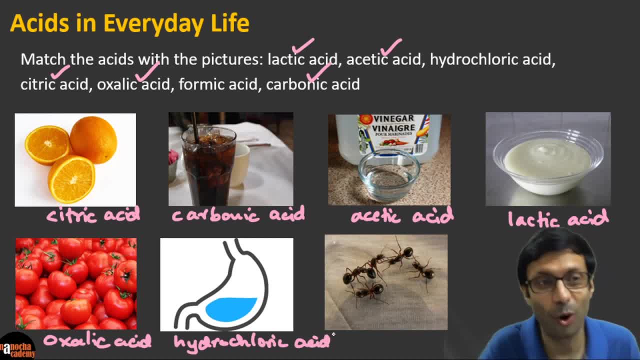 So you guys are awesome. You know all the acids in your everyday life. And guys, this last picture, can you see the ants there? Right? So you know that when the ant bites, okay, if the bite of the ant stings us, and that's because it injects some acid in us, right? Absolutely correct. And that's the answer is formic acid. Because I think in Latin, ants are called formica, right? So it's based 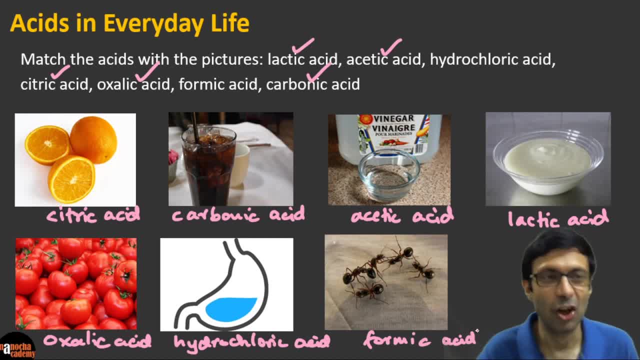 on that. So the sting of ants contain formic acid. Superb. Excellent answers. You guys really know your acids. And if you haven't got some of these, do learn it up because it's important to know which is the main acid present in these things. Okay. Now let's go on to this question. So as you 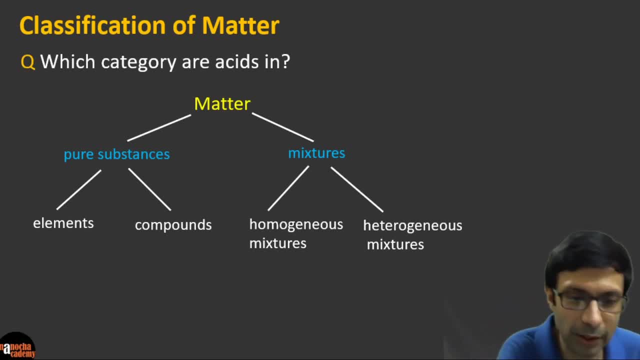 can see here, we've got that matter can be classified based on its chemical properties. So based on chemical properties, we can divide matter into pure substance or mixtures, right? And 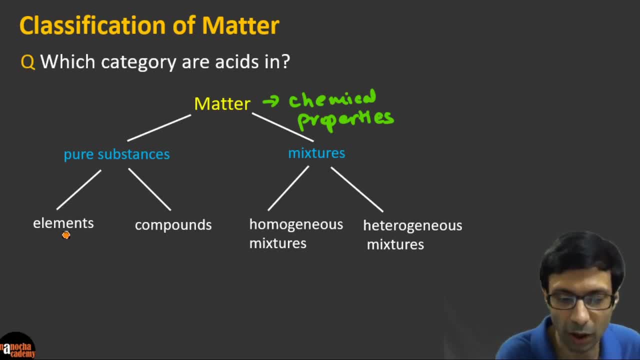 pure substances further can be divided into elements and compounds, and mixtures can be divided as homogeneous or heterogeneous mixtures. So now the question is, in which category out of all of these that you see here are the acids in? Since we are talking about acids here, right? So what are the acids in this chart? Okay. So some of you are saying pure substances. Some are saying elements. Where do you think I should put acids here? Homogeneous. Okay. So think carefully. This 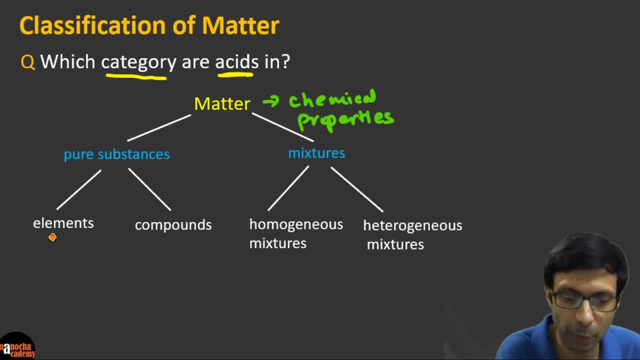 is very important. You should know which category. So by category, I mean the four at the bottom, right? So is acid an element or a compound, right? Which is under the pure substances, or is it a homogeneous mixture or heterogeneous mixture? And here we are talking of the pure acid, not mixtures. So what do you think is the correct answer here? So absolutely right. Acids fall under the category of compounds. Okay. And in fact, this chapter, which is on acids, bases, and salts, all of these guys, acid, bases, and salts, they're all examples of compounds because these contain more than one 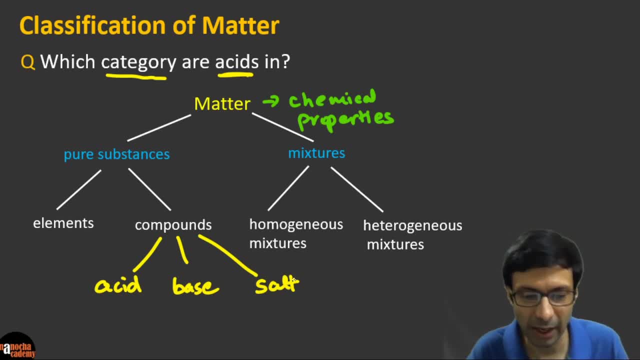 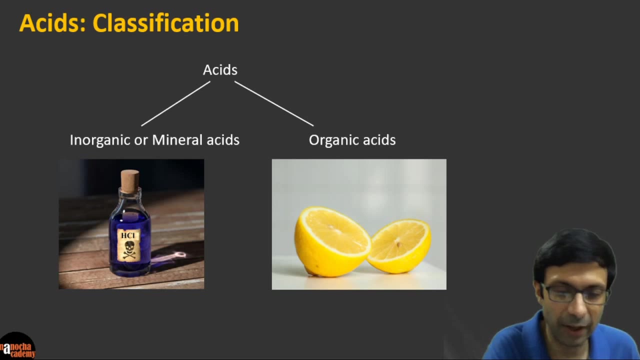 element. Okay. So absolutely right. Compounds is the answer. And we are going to talk about the acids in this video. Okay. But remember they are under compounds, which is under their pure substances. Excellent. So now, since we talked about acids here, right? We can, which came under 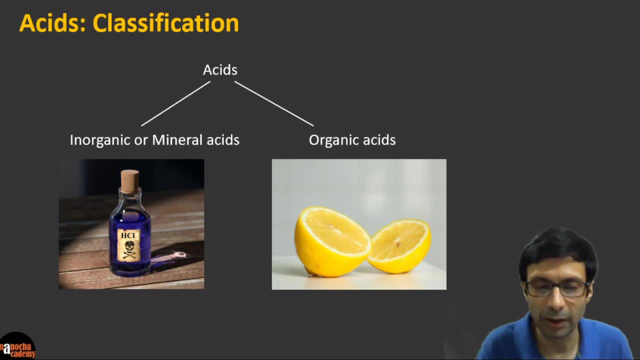 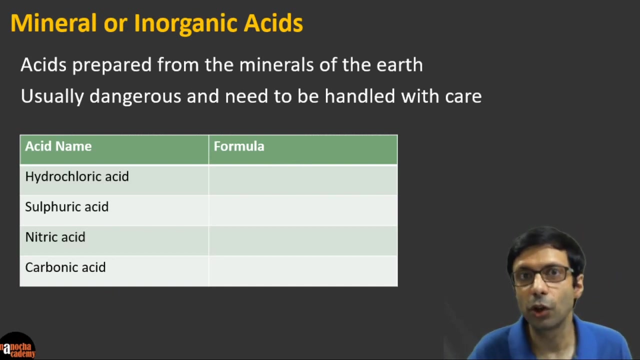 the compounds category, we can further classify acids into these two categories. So can you see guys, it can be inorganic or mineral acids and organic acids. Okay. And we are going to talk about these two categories. So acids can be divided as inorganic or organic and inorganic. Another word is mineral acids. Okay. So what is the definition of mineral or inorganic acids? These are the acids 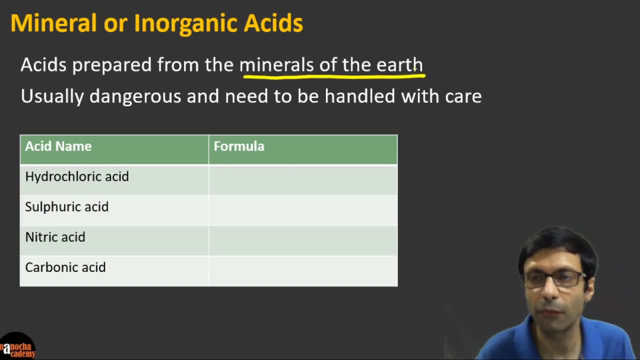 that are prepared from the minerals of the earth. Okay. So they're found on the earth's crust, or they're prepared from those minerals. And these acids are usually dangerous. Okay. So 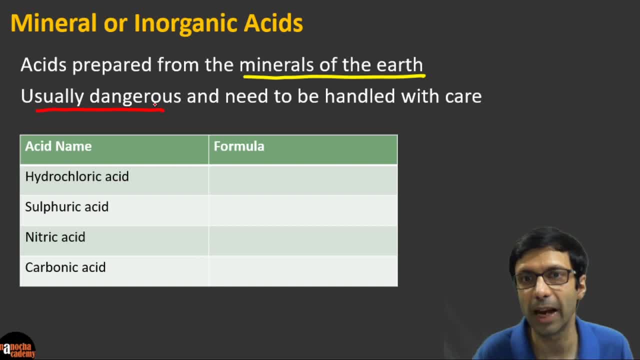 most of the mineral acids are usually dangerous and they need to be handled with care. 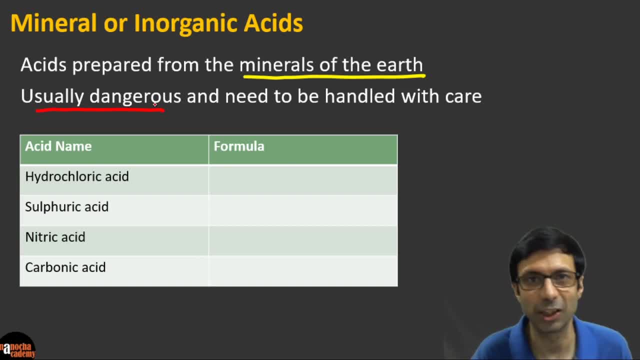 All right. And here I have some examples of mineral acids for you. So let's take a look at this acid. The first one is hydrochloric acid, right? So hydrochloric acid, can you tell me what is the formula of hydrochloric acid? So let's write down these formulas because you need to know them in this chapter. Excellent. It's HCL, right? Hydrochloric acid is HCL because it's made of hydrogen and chlorine. And you guys know that valency of hydrogen is one, chlorine is one. So to form the compound, since acids are compound, you do the crisscross, you're going to get HCL. Okay. Right. And the next one, yes, someone is saying that HCL is present in the stomach. So yes, these are general classifications. So it doesn't mean it can only be found on the minerals of the earth. We know that HCL is produced in our stomach as well, but this classification of inorganic, organic is a rough one, but primarily it can be obtained from hydrogen. Okay. What about sulfuric acid? What is the formula? So very good. The correct answer is H2SO4. So how do we know that? Because it's made of hydrogen and sulfate and sulfate has the valency too. So it's H2SO4, not HSO4. Okay. Next guy, what is the formula of nitric acid, which is also a mineral acid or inorganic acid? Very good. It's HNO3. It's made of hydrogen and nitrate. Okay. 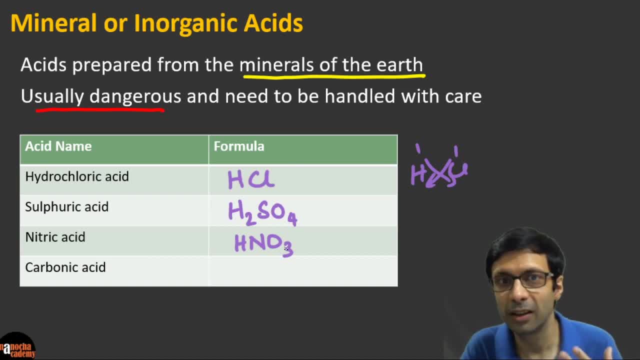 And what is the formula of the acid that is found in the sodas, right? In the colas, the carbonic acid, what is the formula? So very good. You guys, it's not HCO3, it's H2CO3. Okay. And how will you remember that? Because guys, you need to learn your valency. Okay. So what is H2CO3? It's, why is it? Because hydrogen has a valency one, carbonate has a valency two. Okay. It's the 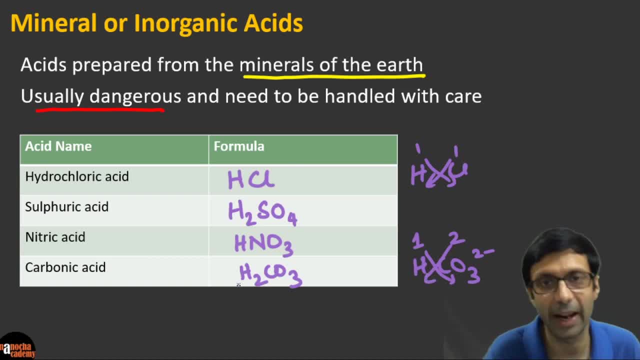 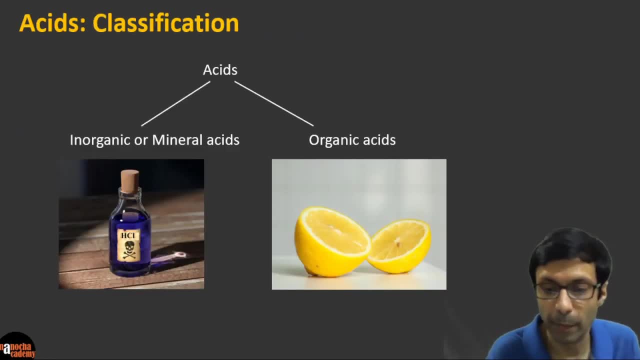 two minus, right? So if you do crisscross, you're going to get H2CO3. So remember these important formulas. And remember we said acid can be divided into mineral or inorganic and organic. So we 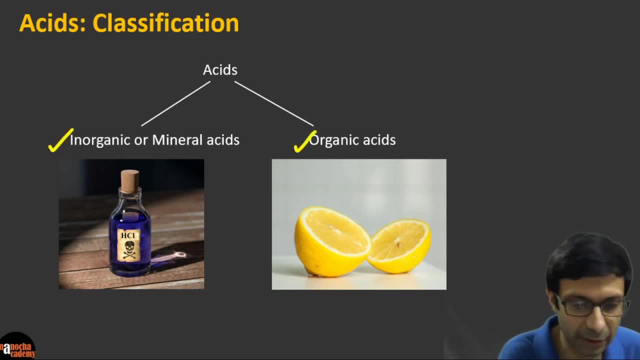 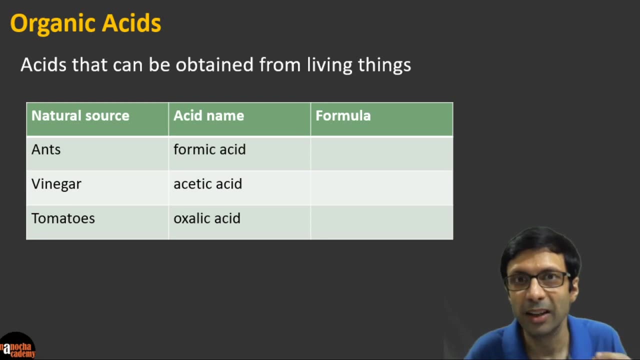 talked about the first category. Now let's look at organic acids. So organic acids are called organic because as you can know from the name organic, that these are obtained from living things. So they can be obtained from living things. Again, as I told, 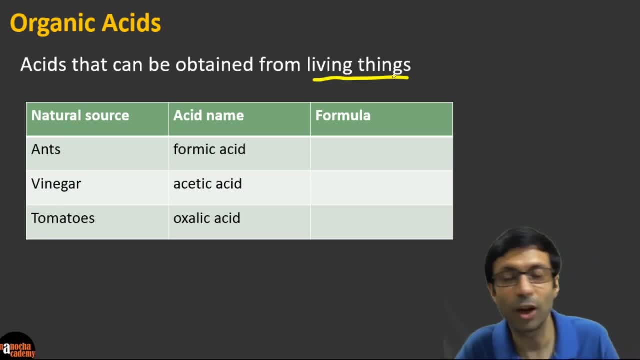 it's a rough classification. So some of you are asking me, when do I come, when do I have these live sessions? It's usually at 8pm and I'm trying to take it every day. You know, I didn't take one on Sunday, but rest of the days I'm trying to have a live session every day. So guys, do subscribe to our channel and click on the notification bell so that you get notified about these live 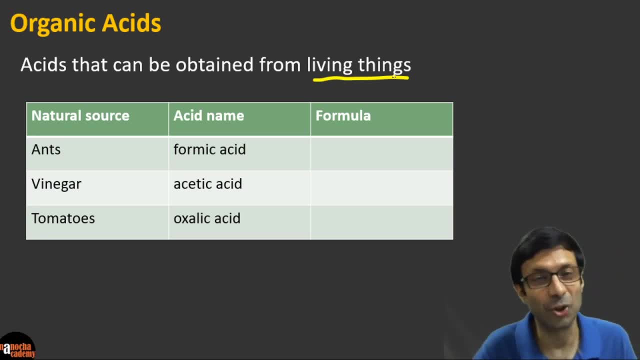 sessions and any new videos we upload. And do remember to share it out with your friends. 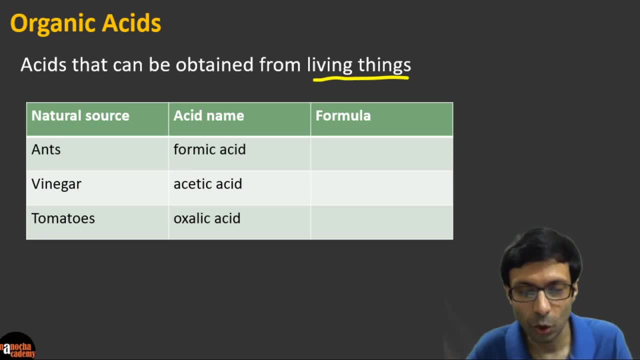 Okay, so let's take a look at these organic acids. So ants, as we said, the sting of ants 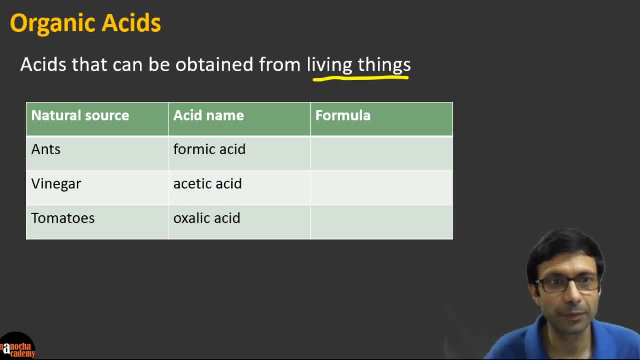 contain formic acid. So do you guys know what is the formula? So what is the formula for formic acid? Does anybody know? Okay, the formula for formic acid is HCOH. Okay, and this is going to 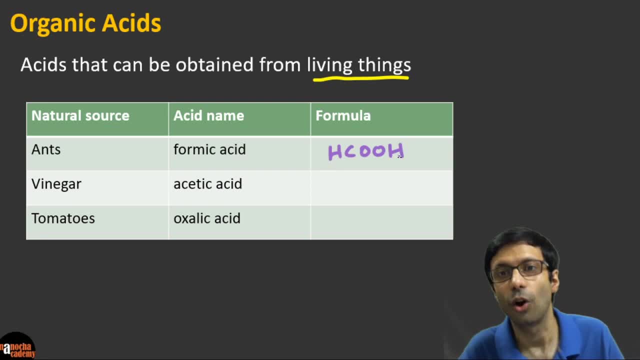 come. So good, I see some of the answers. And you're going to be seeing this in the organic chemistry chapter, the chapter on carbon and carbon dioxide. So let's take a look at these 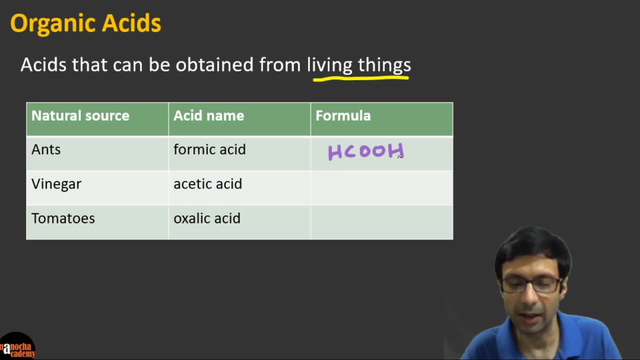 and its compounds. Now the next one, vinegar, acetic acid. Do you know what is the formula of acetic acid? So this one is going to be, it's very similar to the first one, except instead of 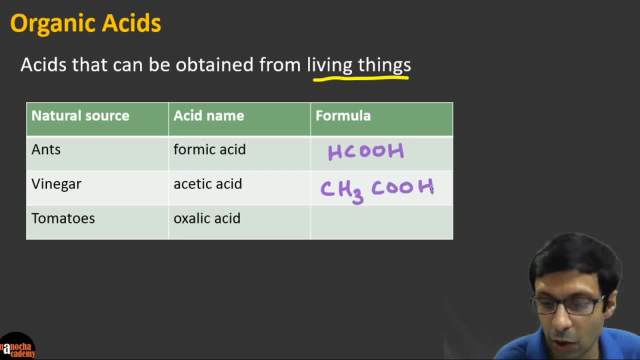 hydrogen, it's CH3COH. Okay, so the vinegar that we eat, it contains acetic acid. Right? And the next one, oxalic acid, the ones that's present in tomatoes. So very good. I see a lot of you know 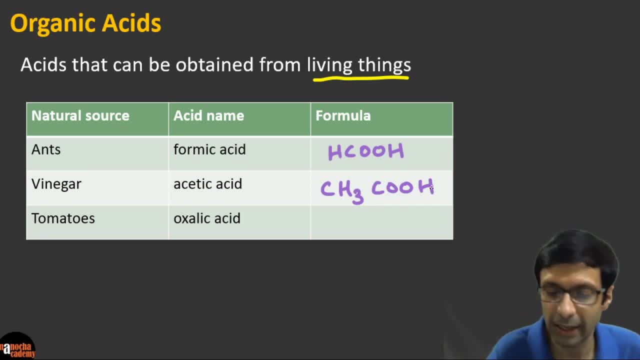 that. So you can remember it in an easy way. It's COOH whole twice, right? So if you work that out, 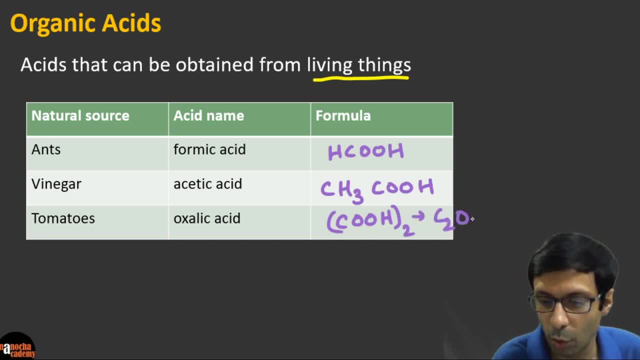 that's going to be C2O4H2. Okay, but easier way to remember that is COOH whole twice. Now one interesting thing you'll notice that these organic acids, they contain the COOH group. 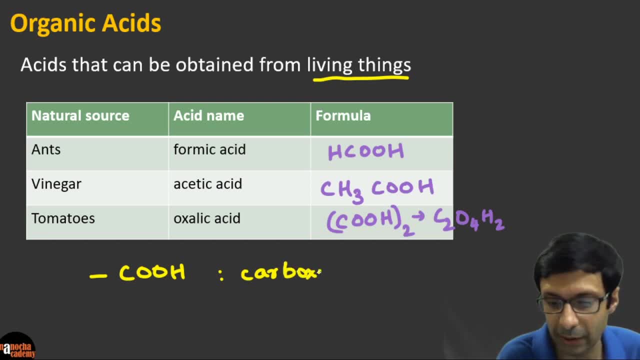 These are known as carboxylic acids. Okay, and you'll be learning more about this in the chapter on organic chemistry or some of you may be knowing this already. So the carboxylic group is called the COOH and the organic acids, they 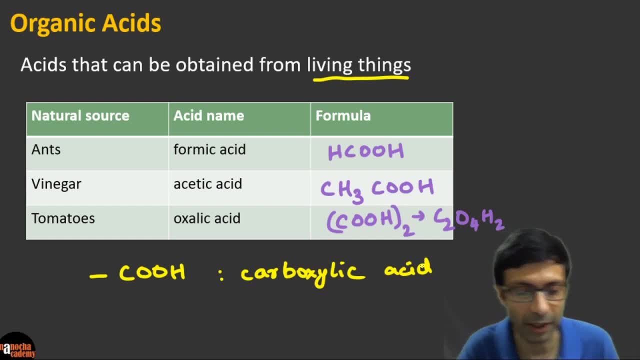 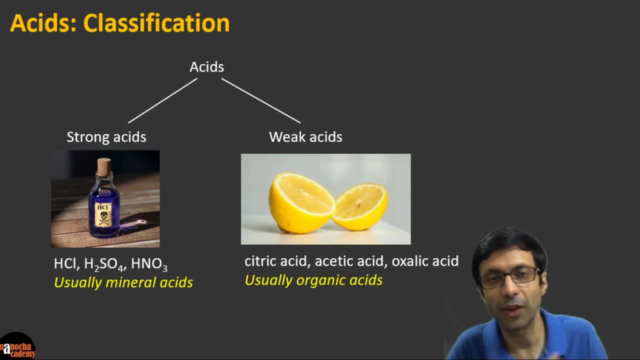 must contain carbon. And not only carbon, they contain the COOH. All right. Now, we talked about classifying them as mineral, inorganic or organic acids. Here's another way to classify acids. We classify based on their strength. Okay. So here you can see we've classified based on the strength of the acid. So we can say is it a strong acid or a weak acid, right? And usually the examples of strong acids are, as you can see here, the HCl hydrochloric acid, sulfuric acid, HNO3 nitric acid, these are 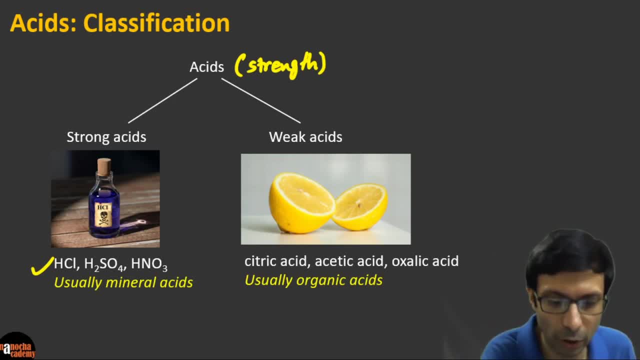 good examples of strong acids and they are usually the mineral acids. So strong acids are usually mineral acids. But there are exceptions in chemistry. 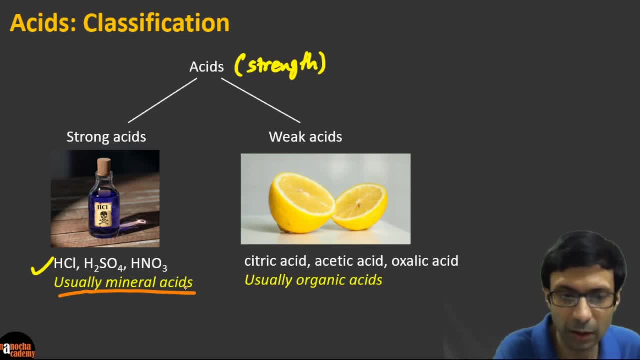 can be mineral acids that are weak. Now let's look at the weak acid examples. So the weak acids are citric acid, acetic acid, oxalic acid. So they are usually organic acids. So what does weak mean and what does strong mean? Strong means they are highly corrosive. These acids are dangerous, right? So the strong acids are usually dangerous because they have a really strong and corrosive nature and the weak acids are not so dangerous. In fact, we eat the weak acid, right? So when you eat a lemon, right, you're eating the citric acid, right? Or when you're having vinegar, you're having the acetic acid, okay? Of course, you shouldn't have too much of it, right? Then you're taking in a lot of acid but it is weak in nature, okay? And our body can take it, we digest it. So usually the organic acids are weak acids and mineral acids are strong acids. Now can you tell me of an exception? Like for example, if we take carbonic acid, right? So the carbonic acid that we talked about, H2CO3, which category do you think it will fall in? So would you put it under strong acid or weak acid? Guys, what do you think? Where should I put carbonic acid? So what do you think is the answer, guys? So carbonic acid, which I told you is present in the sodas, right? 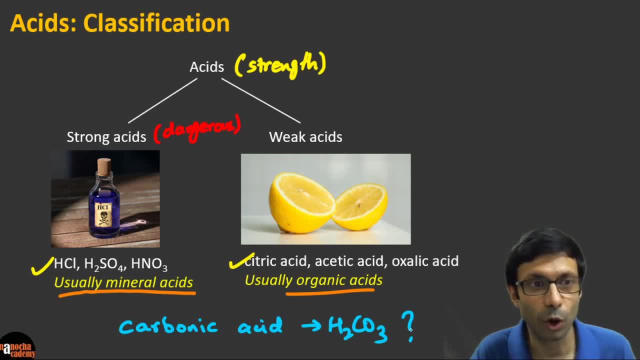 In the drink, the soda drink. So good. So the answer is it's a weak acid and you can remember that because when you drink the colas or the sodas, you are able to drink the acid, right? So it's definitely not a strong acid. So that's an easy way to remember that the carbonic acid falls under weak acids, okay? So it is carbonic acid is a weak acid but it is a mineral acid. So it is an exception. So carbonic acid is actually a mineral acid but as you can see, it's a weak acid. So this classification that strong acids is usually mineral and weak acids are usually organic, right? So there's the word usually, there can be exceptions there, okay? 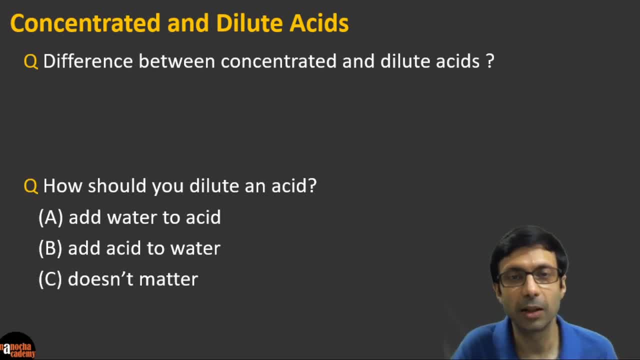 Now here's another interesting question for you. So you might have heard these terms or when you go to the chemistry lab, you hear these terms, right? There's dilute acids and concentrated acid. 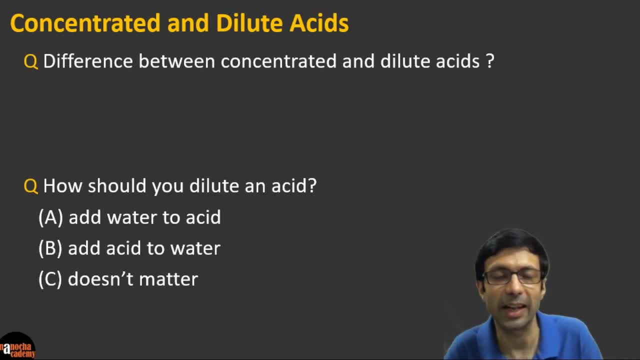 So can you tell me what is the difference between concentrated and dilute acid? 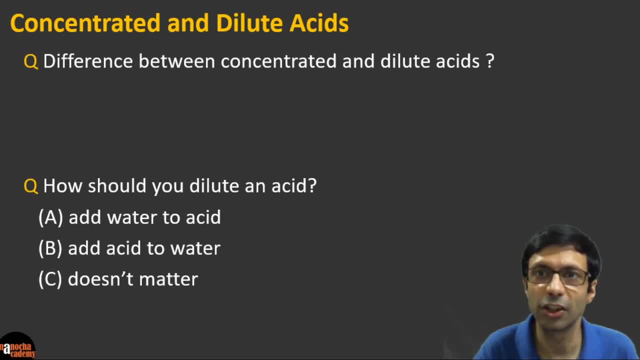 Okay guys, so can you tell me what is the difference between concentrated and dilute acid? So here's the first question, 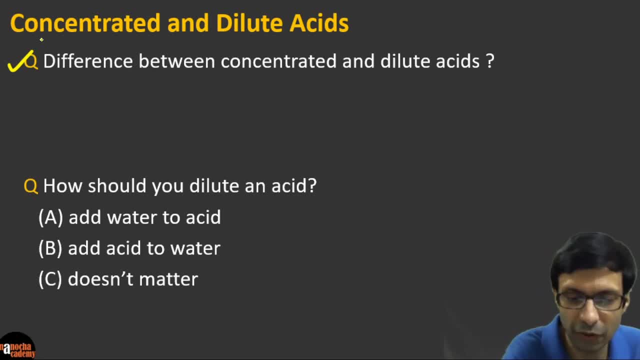 right? So what is the difference between concentrated and dilute acid? 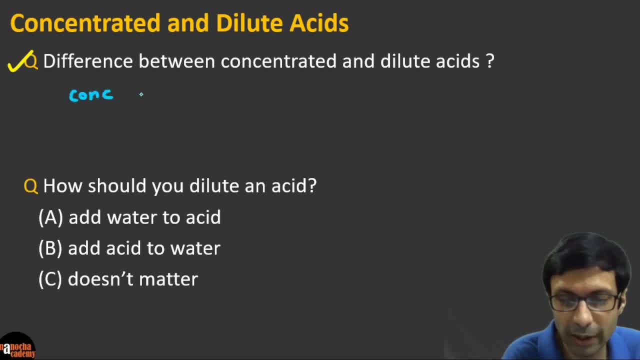 So we know that the concentrated acid basically has less water, right? Or no water, right? So usually it has less water and when you add water to it, you get the dilute acid and on mixing this, it generates heat, okay? So what is dilute acid? Dilute acid is simple. It contains more water, less acid, okay? So the meaning of dilute acid is there's more water and less acid, right? And concentrated acid is the opposite, more acid, less water, okay? Simple. 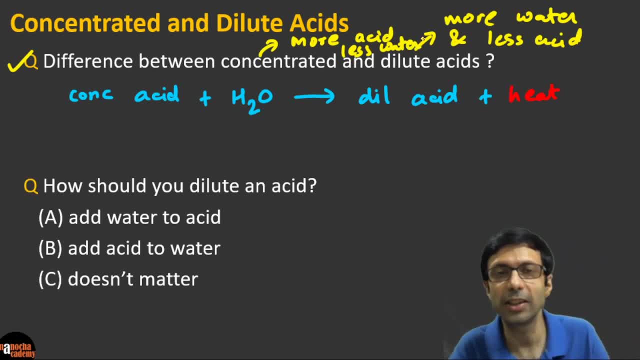 And so how do we go from concentrated to dilute acid? Very simple. We need to add water as you can see in the equation here, right? So to go from concentrated to dilute, you just add water. 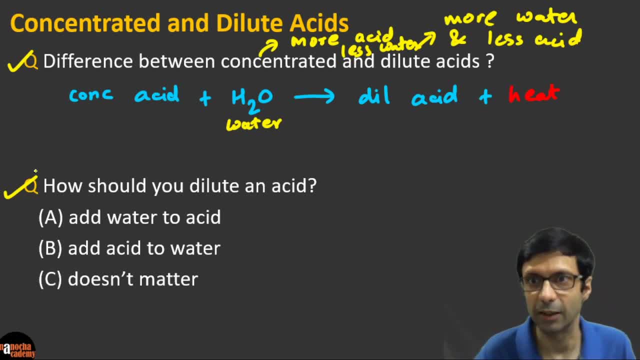 Now the interesting thing is, how should you dilute an acid? So here I have this question. So here are the three options. Should you add water to the acid? Should you add acid to the water? Or it doesn't really matter? So what do you think is the correct answer here? 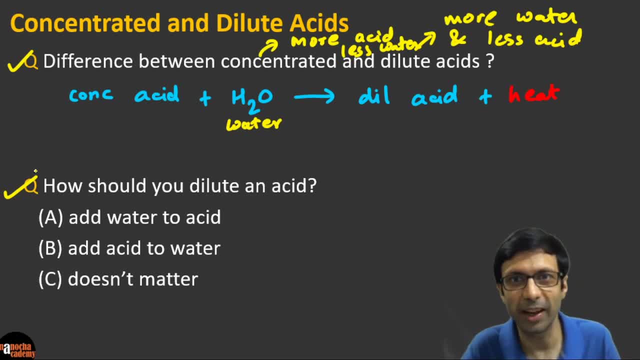 Okay, some of you are saying A, some of you are saying B. So guys, what do you think? So when you dilute an acid, right? What should we do? So let's say this is our beaker here. Okay. 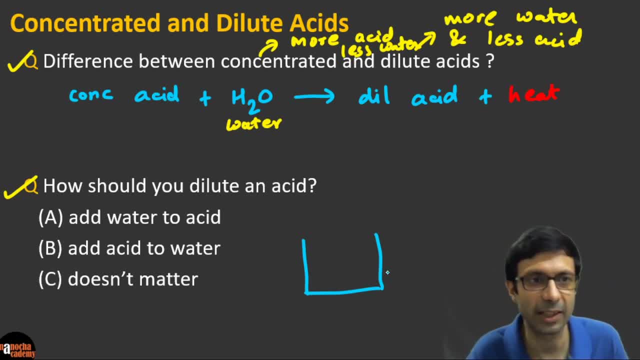 be adding acid to the water or water to the acid or it doesn't matter the correct answer 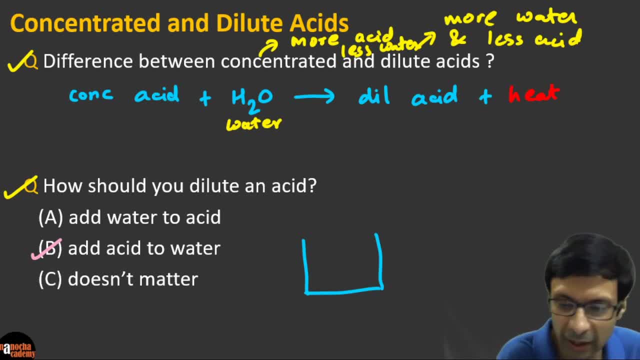 is B okay and we will understand why so let's say we are taking a beaker full of water and we are going to be pouring the acid into it okay let's say this is the acid so the acid is going to be gently poured into it and we are going to be stirring this beaker constantly with the help of a stirrer here right and why do we do that because if you look at the equation on top the important thing is this is an exothermic reaction it produces a lot of heat okay so if you add water to the acid so if we did the first option which is not the correct answer if we did this option then the dangerous thing is because if there's a lot of heat produced if this beaker contained a lot of acid that acid can spurt out okay because a lot of heat is concentrated so the acid is going to spurt out and you it may hit your face or your hands so that's dangerous but if you add acid to the water slowly water has this property of absorbing the heat easily it has a high heat capacity so the water can easily absorb the heat and the heat gets distributed in the water because we are stirring it so it's less dangerous so guys this is a very important question it comes in the exam a lot so you should dilute an acid by adding acid to the water. 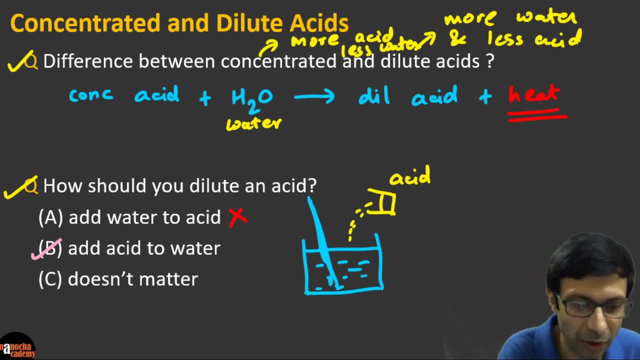 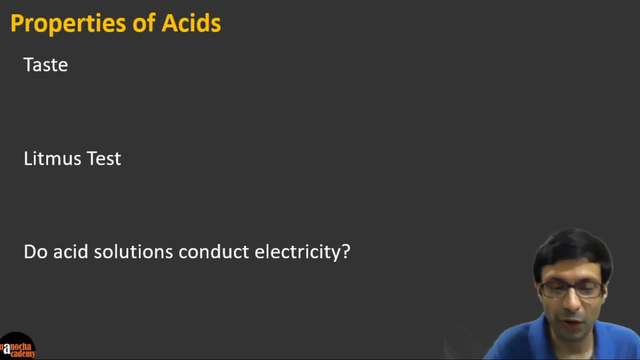 okay guys so please remember this really important point excellent now let's move on to the properties of acids so the first question is pretty easy i'm sure you know it what is the taste of the acid so 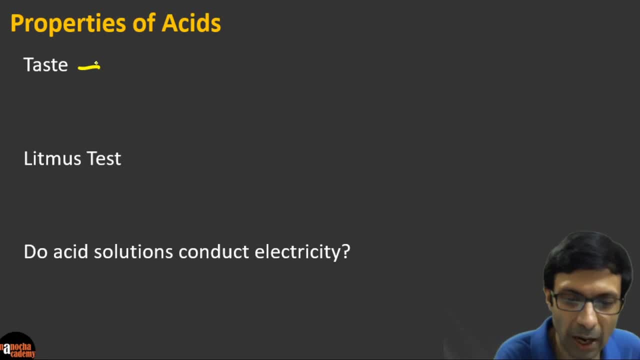 what should i write here so acids have a dash taste what taste excellent i see the right answer 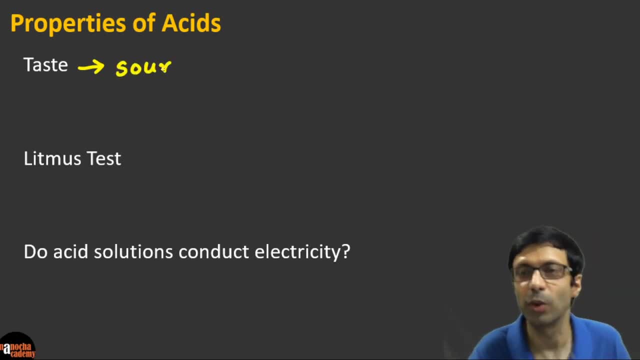 here so you know acids have a sour taste because when you taste lemon you taste an orange it has a sour taste because these contain citric acid so of course there are these mineral 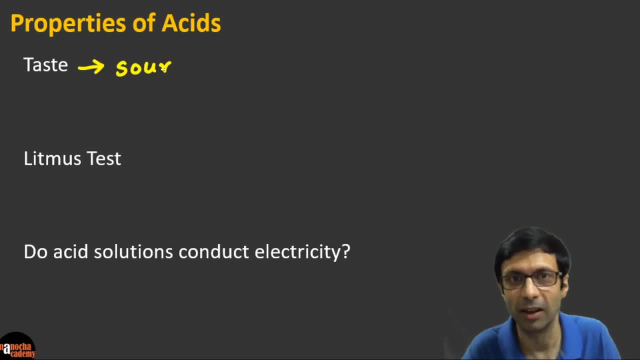 acids or dangerous acids which you should never taste because they are highly dangerous that will burn your tongue but general we say the acids have a sour taste okay very 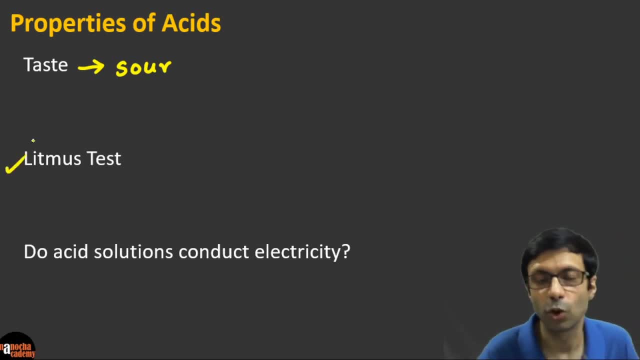 good now let's talk about the next point the litmus test so when you do a litmus test on acids does the red litmus turn blue or the blue litmus turn red or is there no change what do you think is the answer here 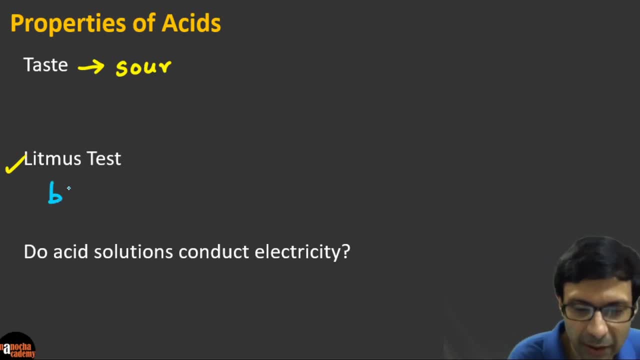 okay so what is the answer here so very good i'm seeing the correct answer the litmus test is the blue litmus turns to red for acids okay so as you guys know the blue litmus turns to red excellent 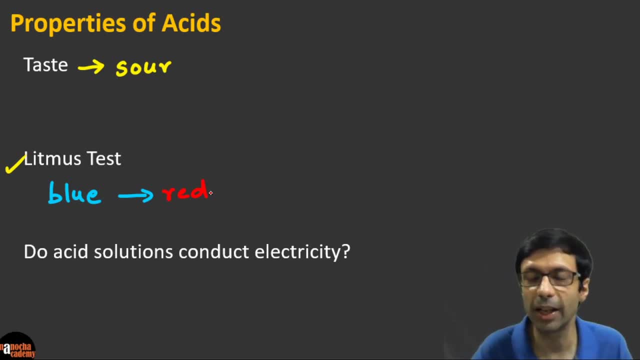 that's the right answer please remember so litmus test is a good test we should not make taste a test for the acids right because the acid can be dangerous so you don't want to taste it when they say how do you test an acid a good way is to do the litmus test now let's take a look at the 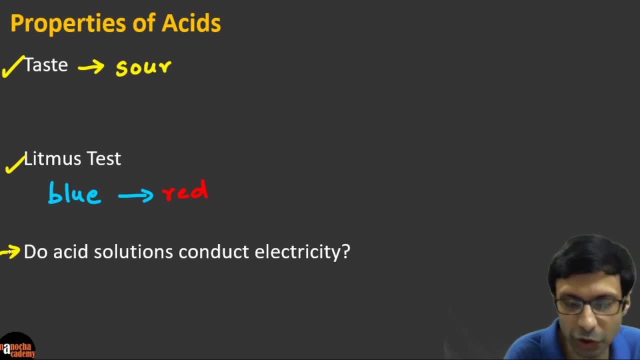 next question so we've done the first two points what about this question do acid solutions conduct electricity 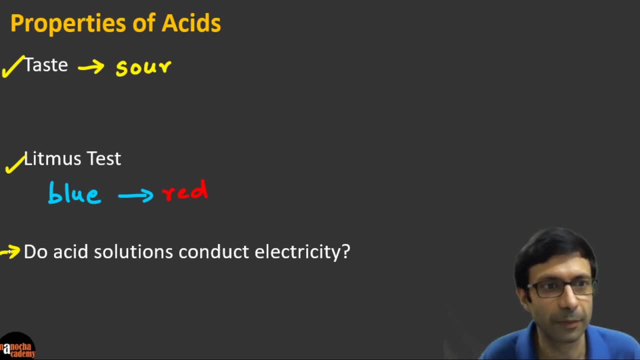 yes or no what do you think okay i see some yeses out there yes they conduct no what do you think is the answer the answer here very good the correct answer is 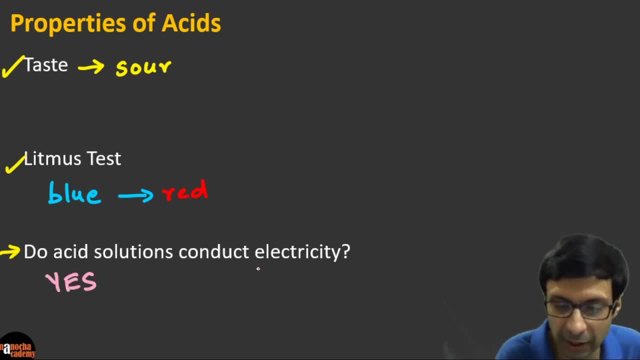 yes so acid solutions are good conductor of electricity and there's a term in science for that they are known as electrolytes because they are good conductors so you can learn this term 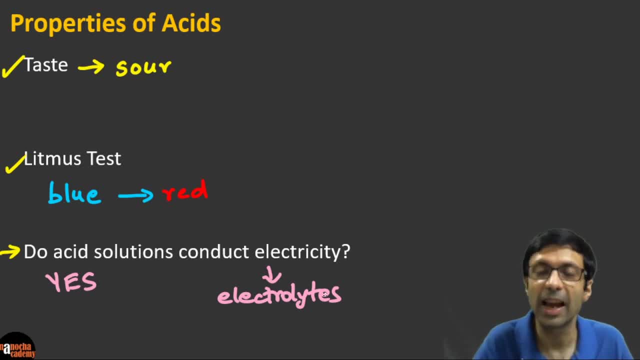 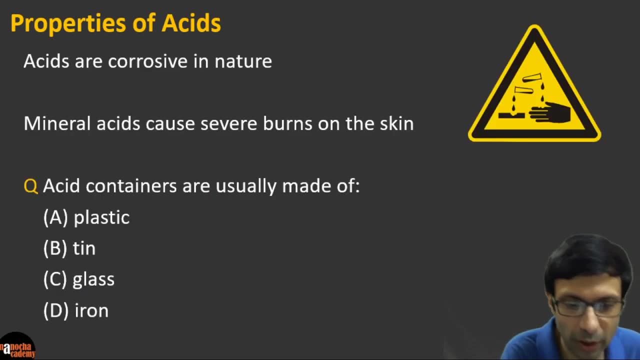 acid solutions they conduct electricity so acid solution means acid mixed in water and we'll see why they're good conductors later on in this class excellent let's move on to the next properties of 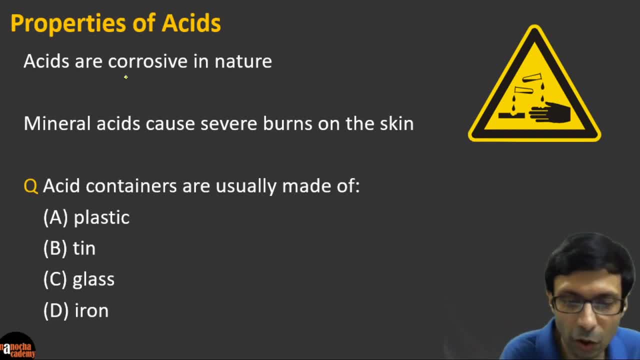 the acids so as we discussed acids are highly corrosive in nature right they're very dangerous they can cause severe burns on the skin so in the lab we should be really careful we should not be casual with when handling acids whether they are dilute or concentrated because 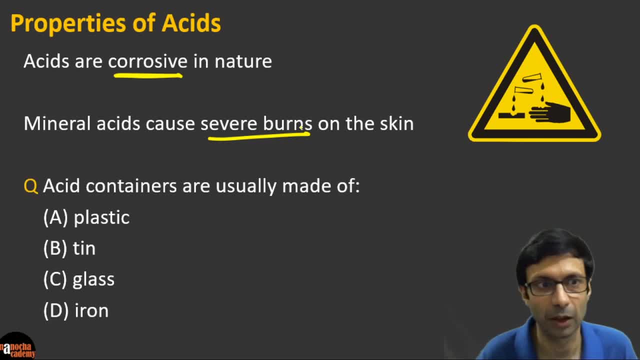 they can be really corrosive and cause burn on the skins okay and now i have this question here for you that acid containers right so where is acid the acid containers are usually made of 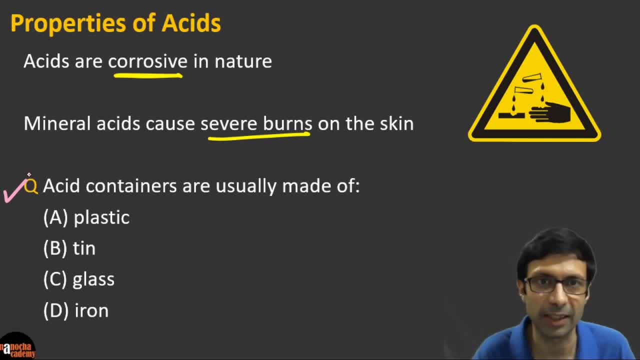 what material so what material is used to store acid and here are our options a is plastic b is tin c is glass and d is iron so guys what do you think and 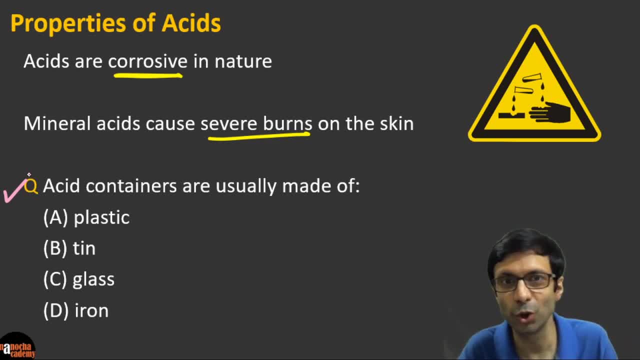 hint is think about your school lab so what material is usually used to store the acids excellent you guys are awesome that's the right answer glass because glass is very resistant 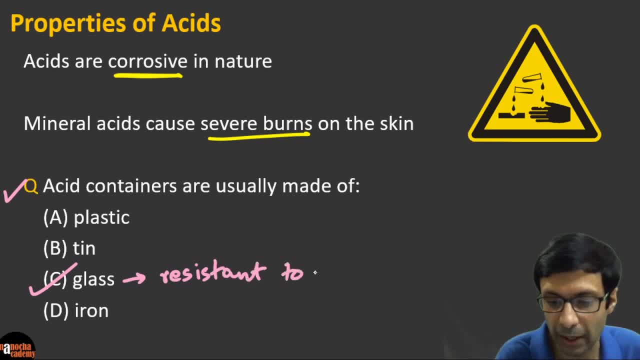 to corrosion right so it is very resistant to corrosion and it's an excellent material used to store the acids and that's why acid bottles are usually made of glass of course you get acid bottles made of plastic also but that's not a good choice right usually because plastic is 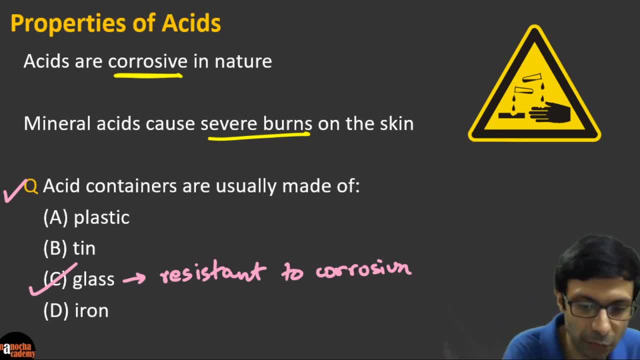 cheaper that's why they do that glass is the best choice because it's very corrosion resistant 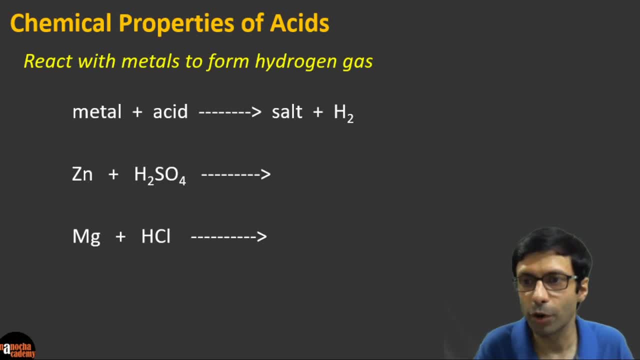 excellent now let's talk about the important chemical properties of acids so this is one very important property which says that acids react with metals to form or produce hydrogen gas so if we write it in equation form we can say metal plus an acid so metal reacts with their acid to form a salt and hydrogen so let's look with the look at this with the help of an example 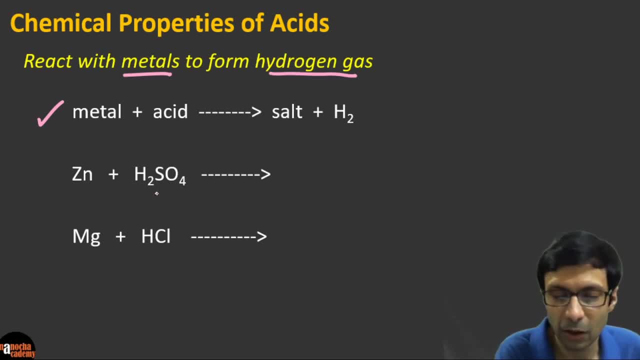 so let's say we react the zinc you know zinc is a metal zed with h2so4 what acid is this sulfuric acid okay and so what do you think is going to happen so we are going to get so what do you think i should write here so go ahead and try it yourself very good i see the right answer you guys have got it it's zinc sulfate plus hydrogen okay and this is hydrogen gas sometimes we mark it with up arrow because the gas is produced okay so zinc plus 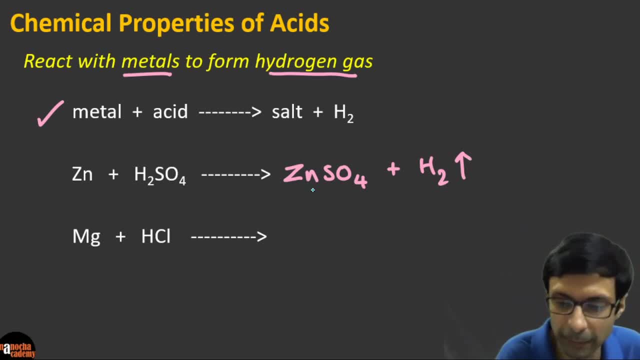 sulfuric acid gives hydrogen gas okay so zinc plus sulfuric acid gives hydrogen gas okay so zinc plus sulfuric acid gives zinc sulfate so this is our salt here okay so that's our salt and hydrogen right and salt 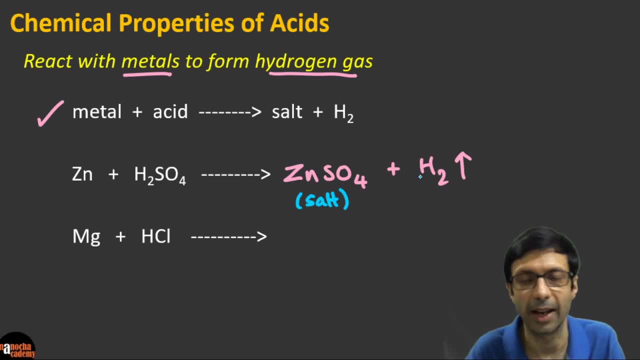 is formed of this cation zinc and sulfate anion right so can you tell me what type of reaction is this so how can we predict that zinc plus dilute sulfuric acid is going to give us zinc sulfate plus hydrogen can you tell me what type of reaction is this and good you guys some of you have tried the next one also we will come back to it. 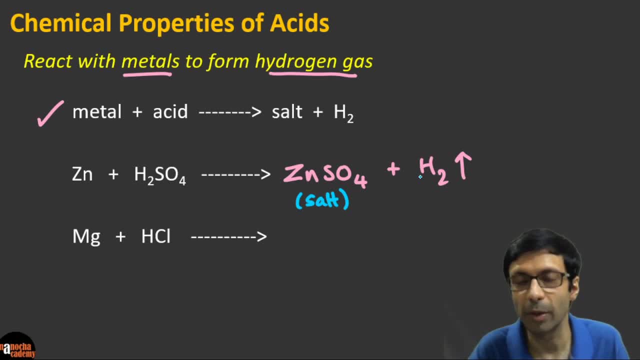 to that so what category based on your types of chemical reactions does this fall into 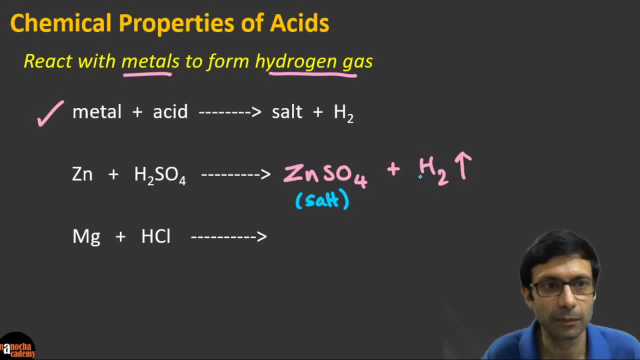 so somebody's asking what is the meaning of corrosion corrosion means the surface gets eaten up right like we say when rusting happens the iron gets corroded so the surface that gets 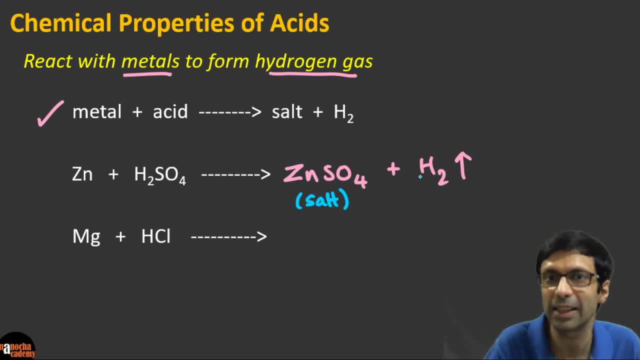 eaten up so acid can actually eat up the surfaces like plastics cane right it just goes and reacts 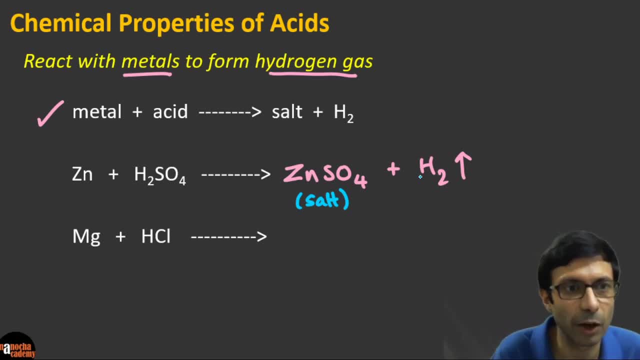 it and removes the surface right so that's the rough meaning of corrosion excellent i see the right answer this is a simple displacement or what is known as single displacement now why is 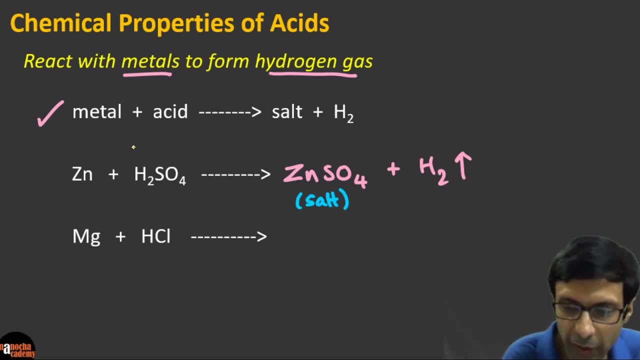 what is happening here why is it called a single displacement reaction so this one let's write that so this is a single displacement right reaction or simply displacement reaction and 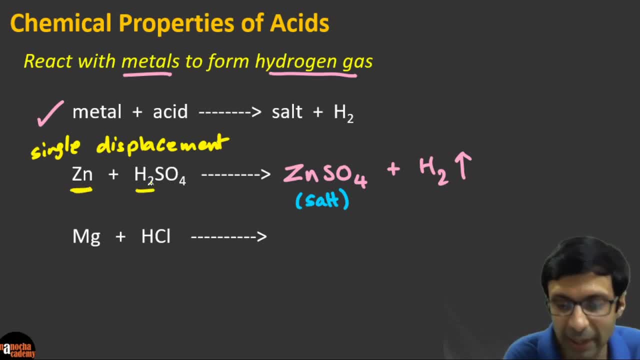 why is that because the metal zinc is displacing out hydrogen can you see it just just 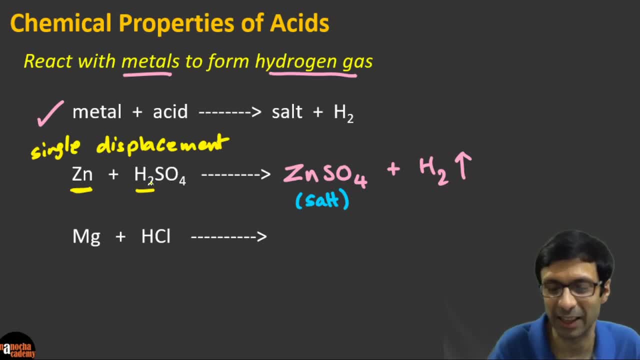 kicks out hydrogen from sulfuric acid and takes its place there and so hydrogen comes out so this is known as a single displacement where you know the reactivity series comes into play and a more reactive element displaces a less reactive so it just tells hydrogen you get out of out of sulfuric acid i'm going to take your place so it's going to be zinc sulfate and hydrogen similarly let's 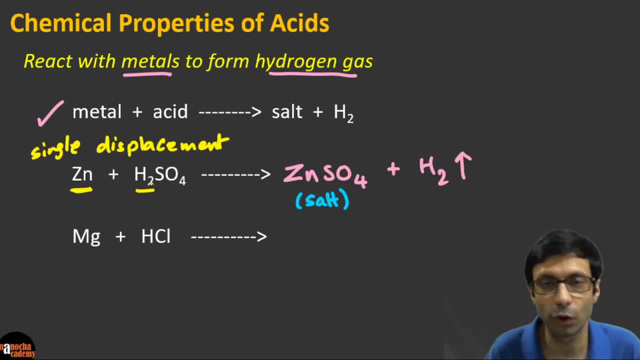 apply this for magnesium and dilute hydrochloric acid so the next one so what do you think is going to be the answer of the second equation 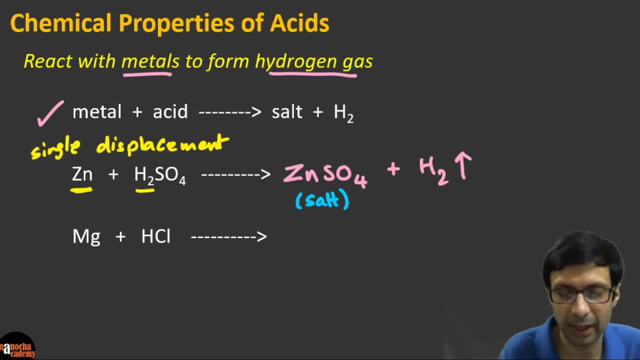 guys so mg plus hcl it's going to be again the same thing can you see single displacement so magnesium kicks out hydrogen okay so it removes hydrogen from here so it's going to be mg so will it be mgcl or mgcl2 mgcl2 very good because it's based on valency right 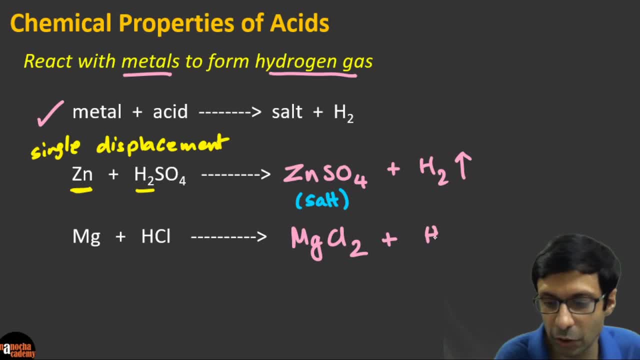 magnesium has the valency 2 and then hydrogen is going to come out okay very good and so this is our solution so we're going to take the hydrogen and dilute it so it's going to take the hydrogen 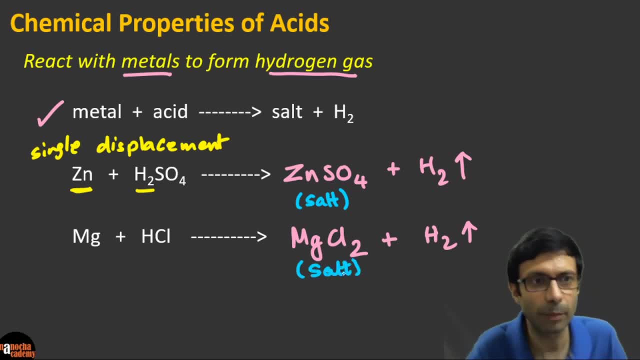 salt and guys is my equation perfectly correct do i need to do something or is the equation good to go 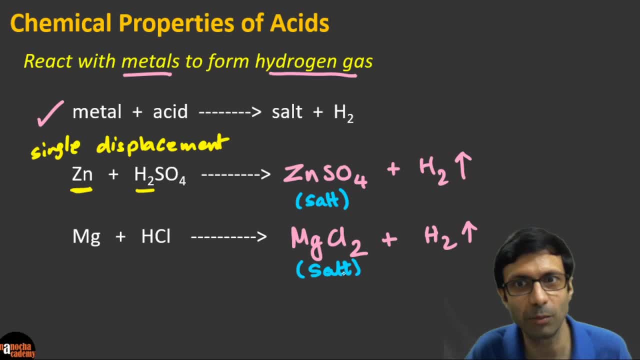 okay so guys what do you think will you give full marks for my equation mg plus hcl gives us mgcl2 plus hydrogen great you guys are great teachers so you caught the thing it's not balanced right 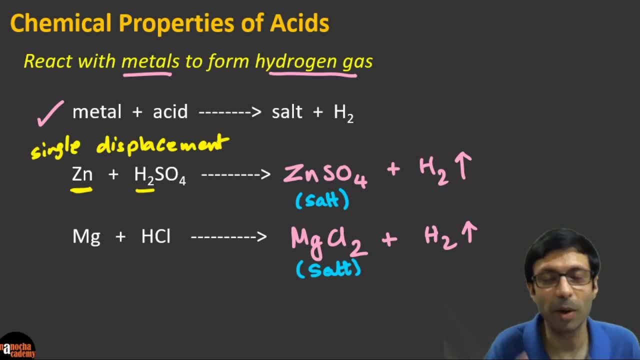 so excellent so please remember in chemistry and i remember i used to walk into the exam reminding 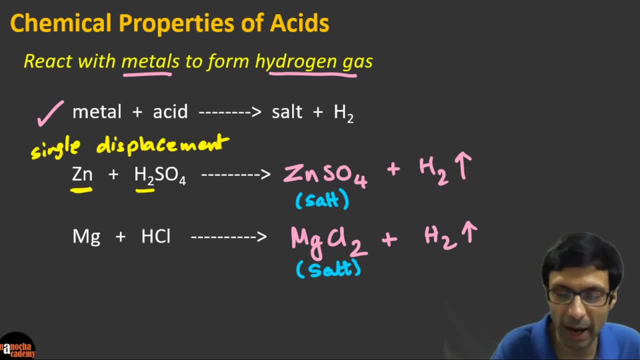 myself to balance the equations right so keep telling yourself to balance and here you can see we need to do plus 2 hcl excellent guys so can you see that a metal when it reacts with an acid 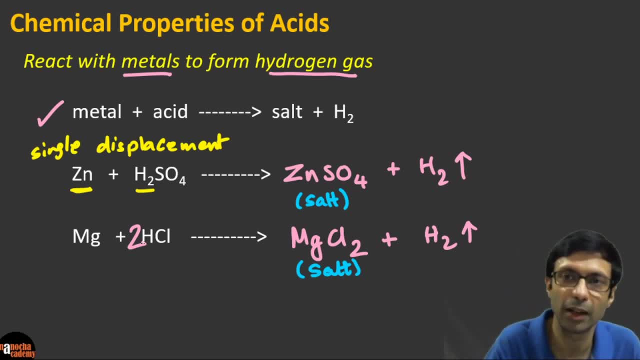 the metal displaces hydrogen so if it's more reactive than hydrogen it will displace it and we get the salt and hydrogen now let's take a look at the next chemical property 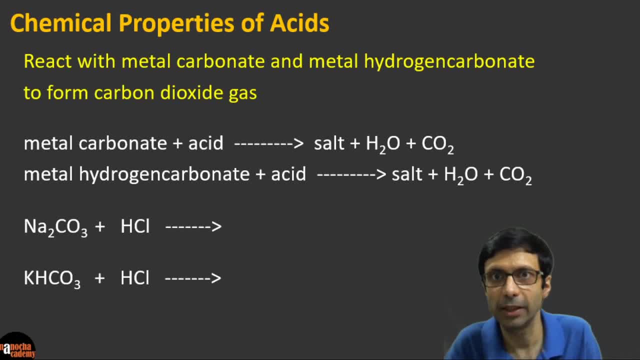 where we say that acids react with metal carbonates and metal hydrogen carbonates and this is also known as so these guys are also known as bicarbonates so you may see this term also 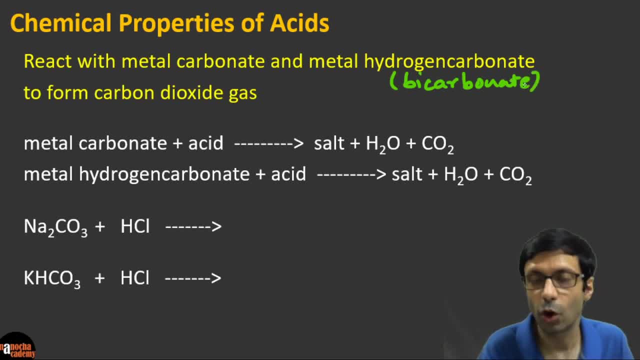 in some of your textbooks and they form salt plus water and now the gas is going to be carbon dioxide okay so take a look at this and there we can you see we've written metal plus metal carbonate plus acid gives us salt plus water plus carbon dioxide and similar equation for hydrogen carbonate so 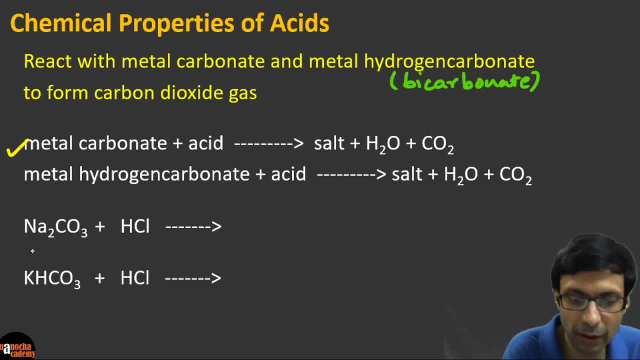 let's go ahead and try it out so let's try this first equation here sodium carbonate plus hcl what do you think we are going to get 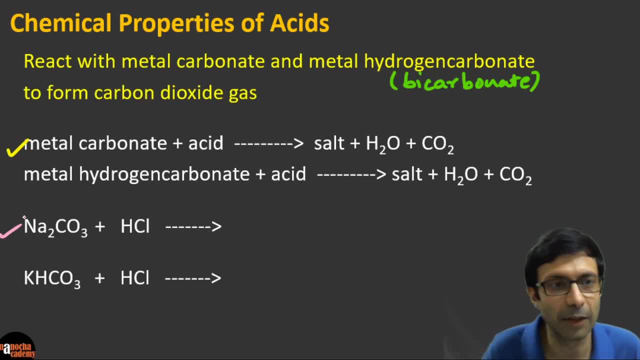 okay guys so apply the concept here that's given so what are we going to get when you do sodium carbonate plus hcl right so let me actually show you a trick of how to predict it one is you can use the rule here but i'm going to show you a secret trick of how to predict this reaction 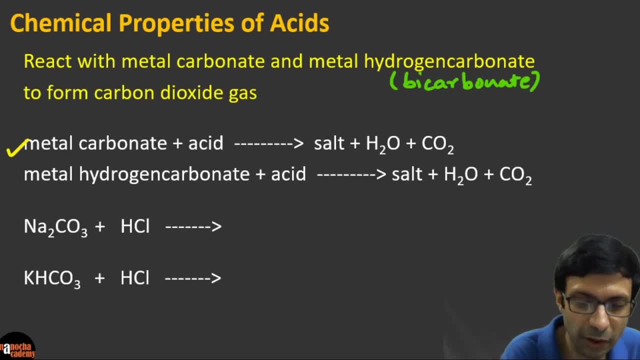 right so let's take a look at this first equation so sodium carbonate we can split it into 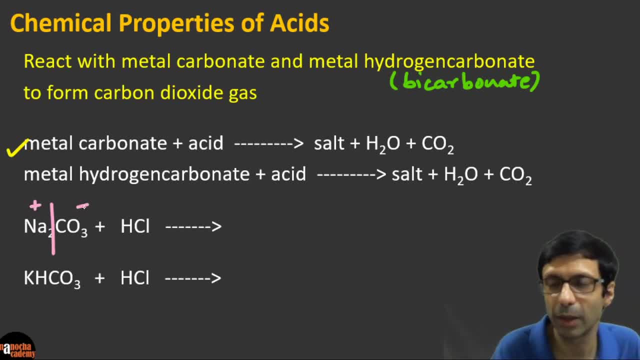 na plus and carbonate minus it's carbonate two minus but i'm just writing minus for now okay and similarly we can break down hcls 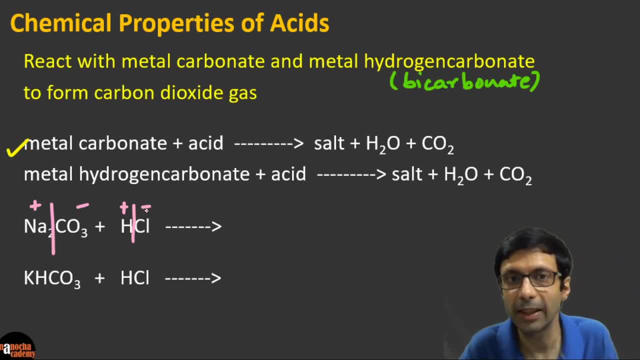 plus minus okay so guys follow me carefully we are breaking these compounds into the cation positive and negative part cation and anion part okay and now what do you think what type of reaction is going to happen here so when you have this cation anion business what type of reaction takes place 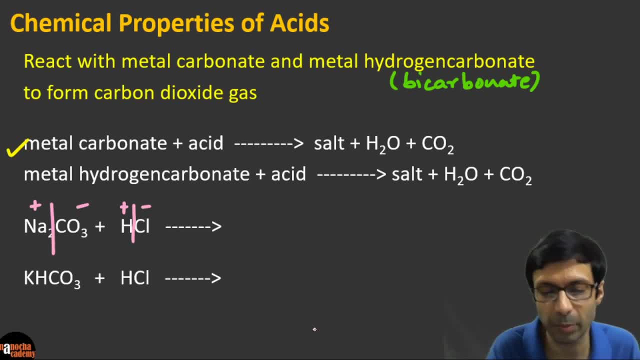 here guys think about it so previous one was single displacement which one will be this type of 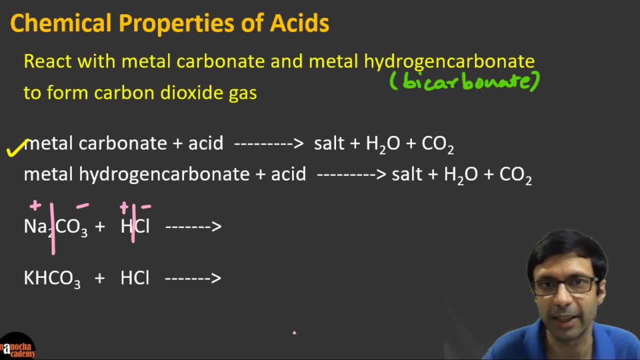 reaction for sodium carbonate plus hcl what do you guys think 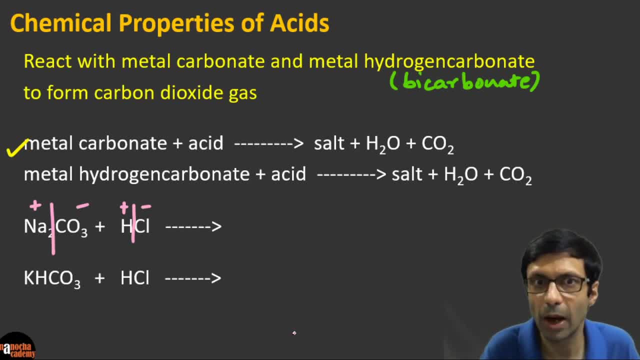 neutralization okay any other type that can form when you have this exchange of ions right so it's not a combination it's going to be an exchange of ions very good i see some of you got the right answer it's double displacement because you can see these cations are going to exchange 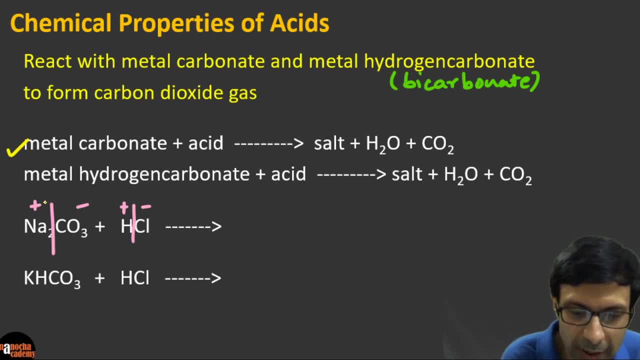 their positions so let's see what does that mean so this guy is going to take this place and hydrogen is going to take the place here so what are we going to get so take a look at this uh trick to predict this reaction so sodium is going to ex exchange places with hydrogen so it's 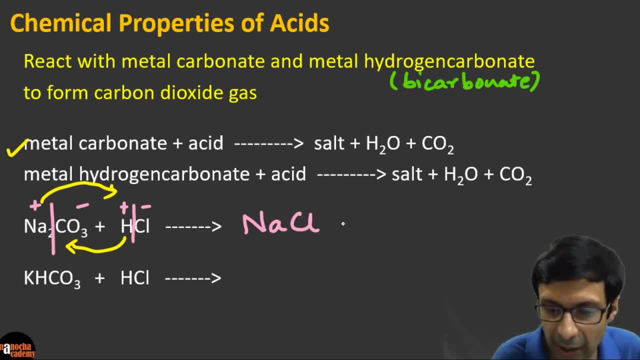 going to be na cl because the valency is one and then we are going to get h and co3 which is going to form carbonic acid h2 co3 so this is very good double displacement or double decomposition is the 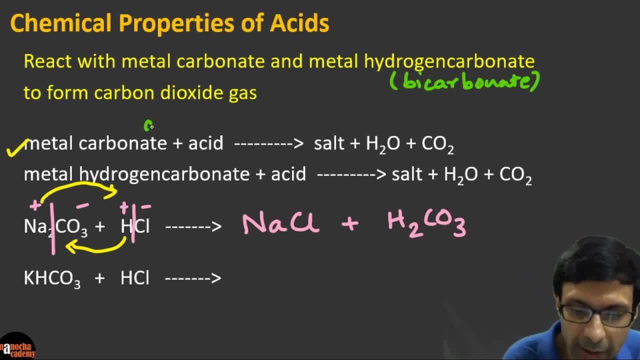 type of reaction here so let me write that down so we are looking at double decomposition reactions in this type so now you can connect your first chapter where you learned about types of reactions 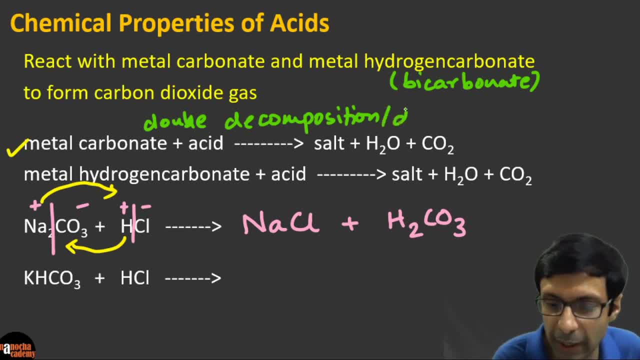 and this one so this is double decomposition or double displacement right and now do you see what's happening necl plus h2 co3 now one very important point carbonic acid is unstable right 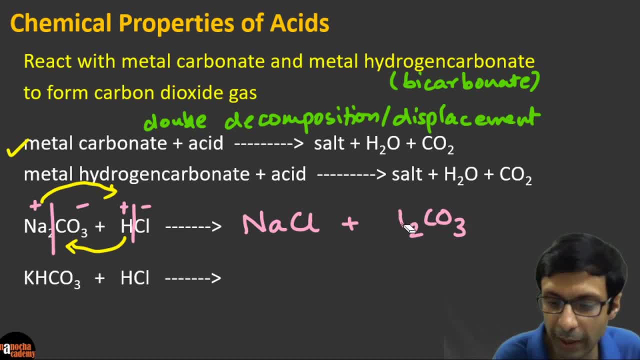 so it's not going to stay as carbonic acid this guy is going to break down into so i'm going to erase this so carbonic acid is going to break down into h2o plus 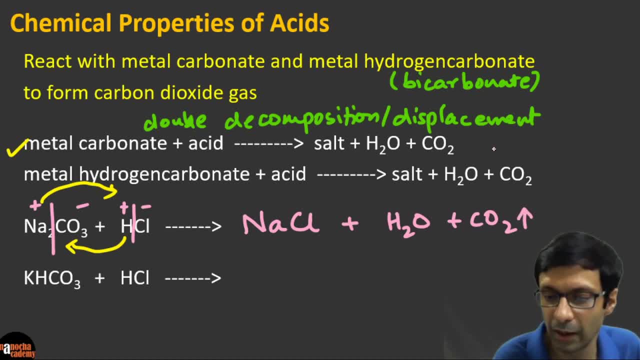 co2 and that's how carbon dioxide is produced okay guys because carbonic acids h2 co3 is unstable 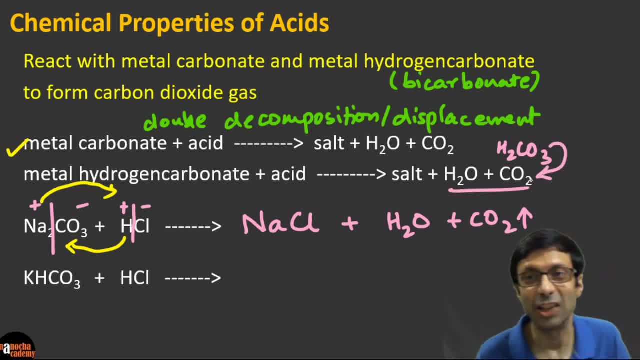 so it breaks down into these two guys okay and so with this help see we predicted our reaction and the last thing we've got left is to balance it so let's quickly go ahead and balance this equation 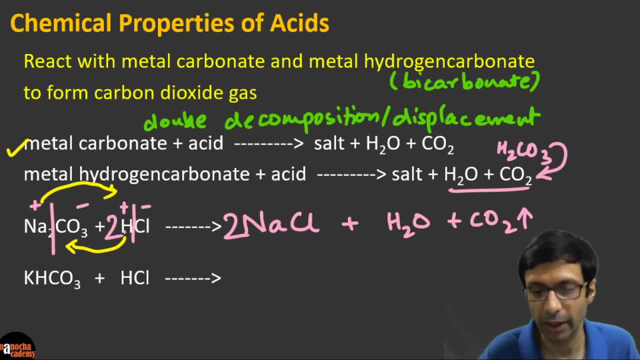 so that's two here right so i think our equation is balanced now excellent now let's take a look at the next one again let's use our secret trick 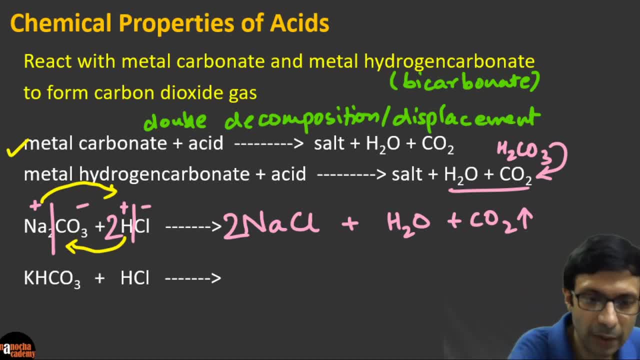 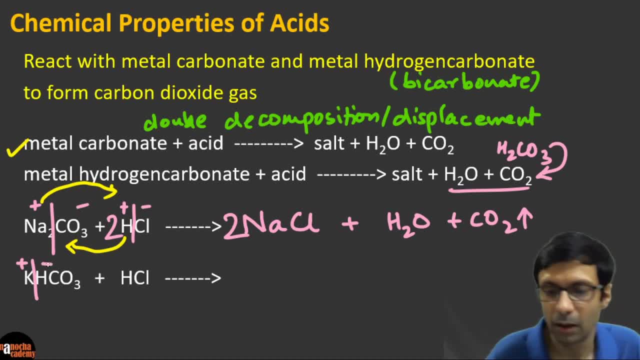 so let's break it down into k plus and the hydrogen carbonate ion or the bicarbonate ion 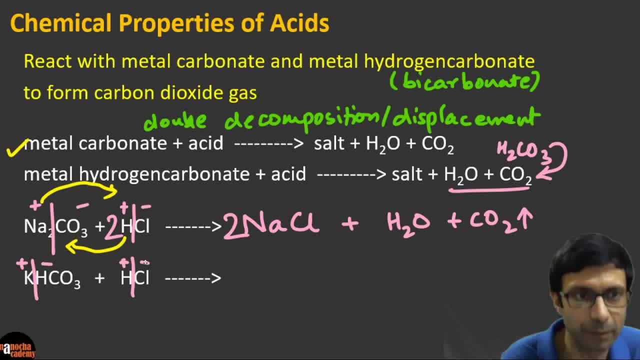 and similarly we'll break hcl into plus minus right so this is a very useful trick for you to understand what's happening so then you won't have to learn these reactions you can simply predict it okay so it's going to be really useful for you and you can see that these guys are going to exchange their positions okay and so what are we going to get it's going to be kcl plus h2 co3 right 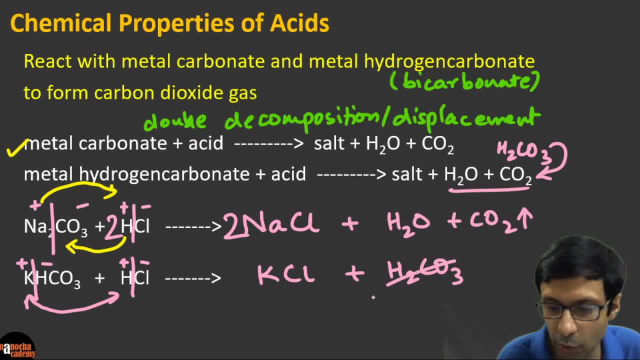 again and remember h2 co3 breaks down into h2o plus co2 okay so don't leave it as uh carbonic acid that's not going to be completely correct and so you're going to get this and i think the equation is already balanced so we get the salt in the first case for sodium chloride the second case 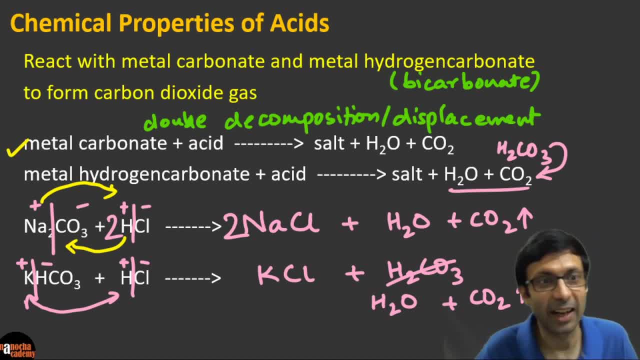 okay and then we get carbon dioxide gas and guys do you know how to test carbon dioxide gas so how do you test the carbon dioxide gas that is produced do you guys know that 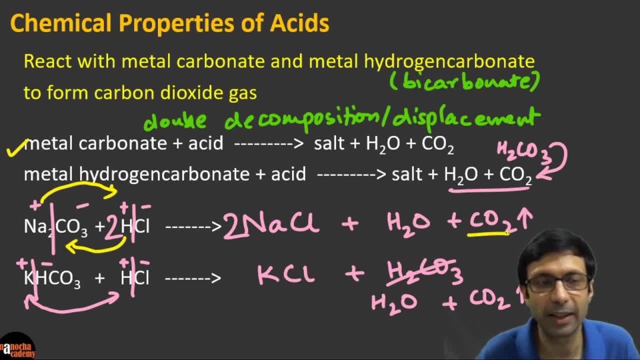 so we've got carbon dioxide being produced here so how do you test carbon dioxide what is the chemical test to test it very good i see the correct answer lime water test right 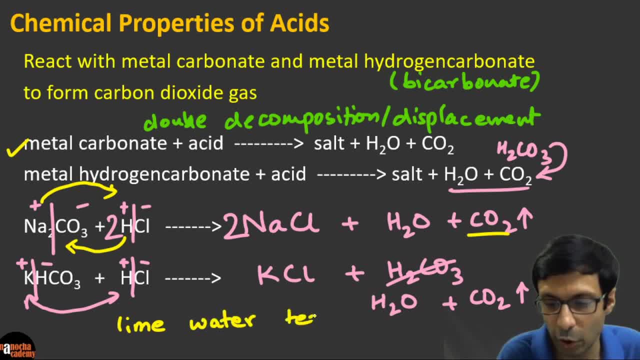 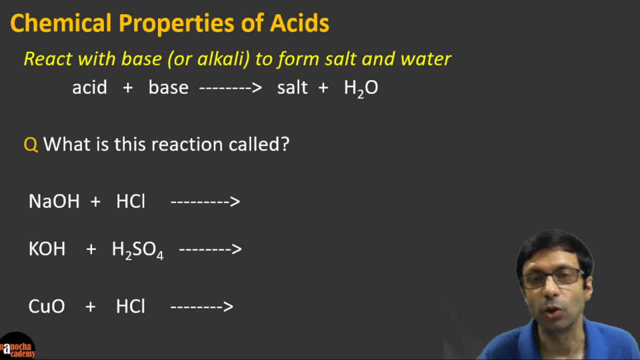 so a lot of you are writing lime water tests in the chat excellent because you know that when carbon dioxide is passed through lime water it turns the lime water milky so this equation can actually be used to test out acids okay very good let's take a look at more properties of acids so this is a 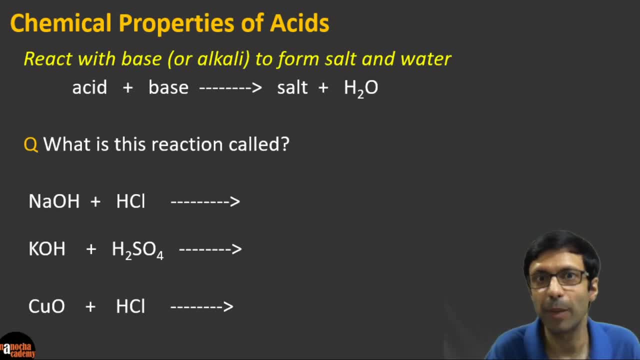 famous property where you must be knowing that acid and base right react to form salt and water 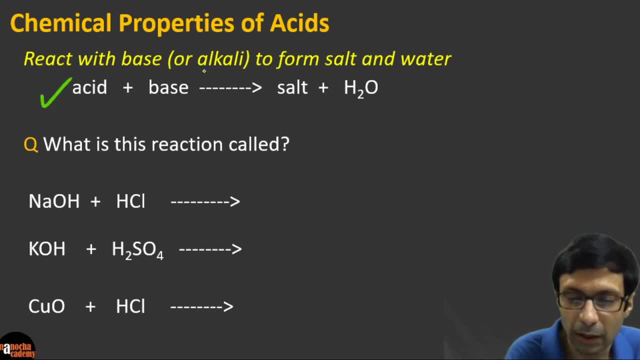 so take a look here and we also say it could be a base or an alkali so guys do you know what is the difference between base and alkali 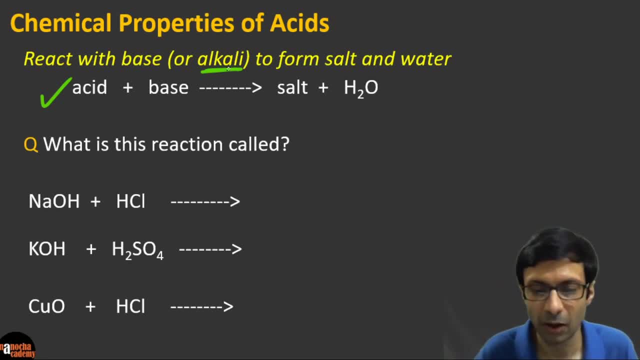 so if you look at this equation we are saying acid plus base reacts to form salt and water here right 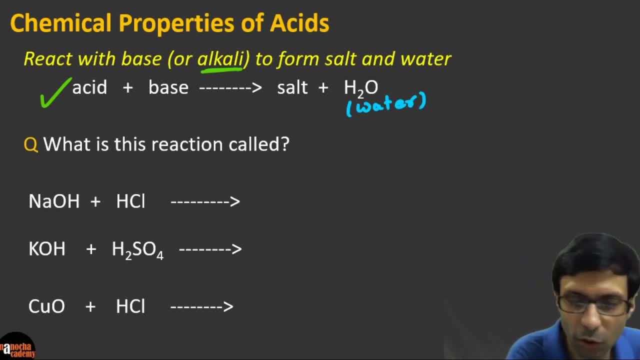 so what is the difference between so as it can react with the base or we can say or it can react with an alkali and very good i see some of you are writing the correct answer the definition of alkali is very simple those bases so let me write it here 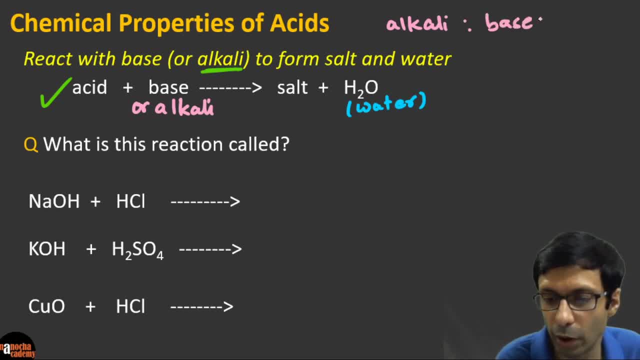 alkali means those bases that are soluble in water so bases that are soluble so bases that are soluble in water 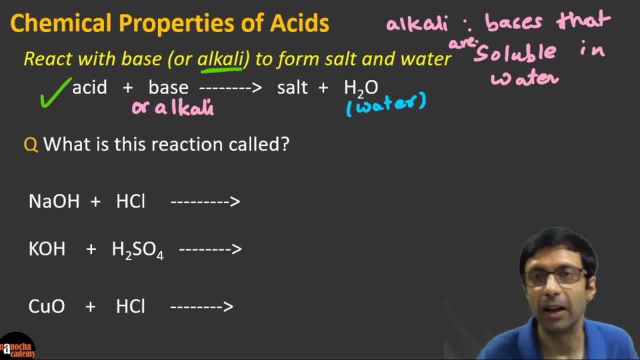 okay so you need to know this right uh the definition of alkali because not all bases are soluble in water and good examples are so from this list can you tell me who are the alkalis so it's going to be sodium hydroxide here is an alkali and potassium hydroxide okay these are the alkalis here copper oxide is not soluble in water and so this is not an alkali so this guy is not an alkali okay so you need to learn the list 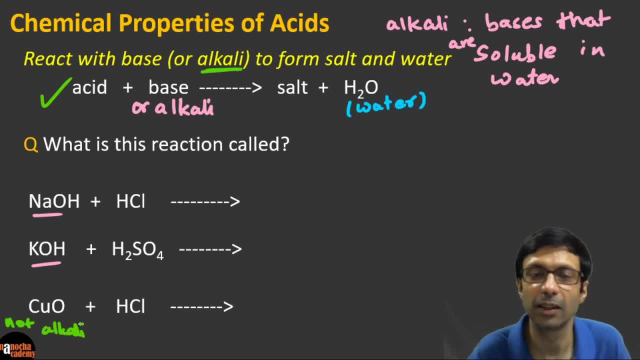 sodium hydroxide potassium hydroxide ammonium hydroxide these are all alkalis okay now let's 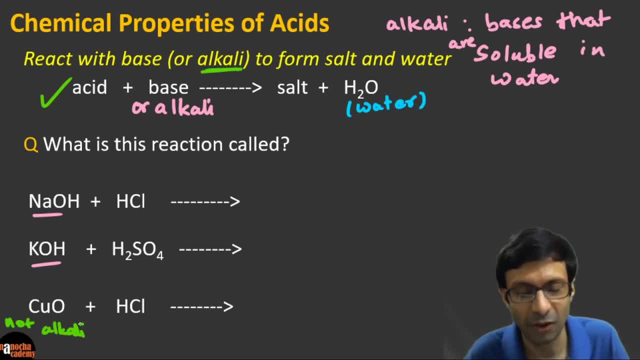 take a look at this important question what is this uh reaction called excellent i see a lot of correct answers so you've given the answer already superb this reaction famous reaction in chemistry acid plus base gives salt plus water is known as neutralization right so neutralization reaction 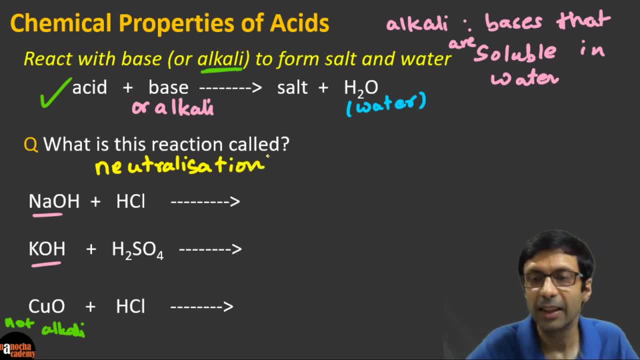 okay so it's called a neutralization reaction because we say the acid is reacting with the base to form salt and water it's neutralizing the base or the base is neutralizing the effect of the acid okay that's why it's called a neutralization reaction and it's a really important reaction 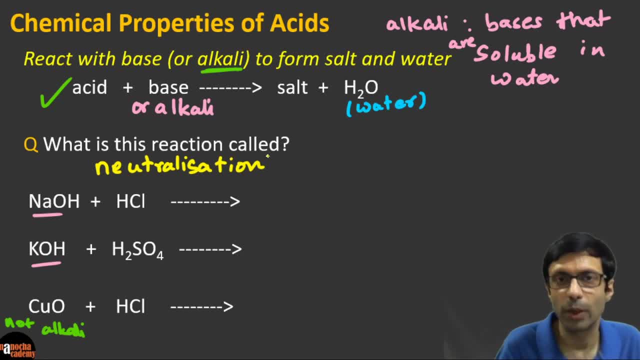 in chemistry so now let's take a look at the first reaction so when sodium hydroxide so this alkali reacts with hydrochloric acid what are we going to get guys so can you try the first equation here so naoh plus hcl what are we going to get and yes that's right neutralization means 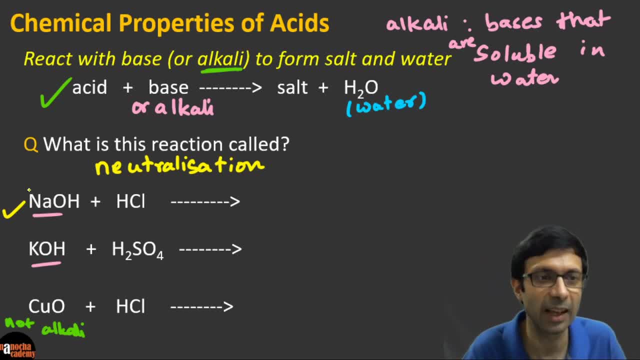 so acid cancels the effect of the base or we can say the base cancels the effect of the acid excellent and a lot of you got the correct answer so the first one is going to be simple sodium chloride right the salt that we eat plus water and again this reaction neutralization fits into which 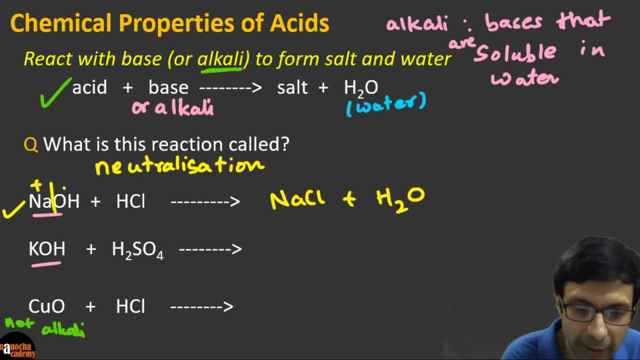 category so if you break this ions plus minus plus minus can you see right so na is uh taking the place of hydrogen it's going to give na cl plus water so can you see that in these cases 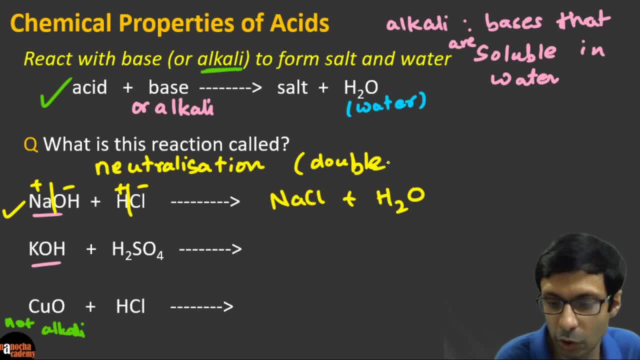 double displacement is happening right so it's of the time double displacement but it's given a special name because it's such an important reaction in chemistry so we call it neutralization excellent it's a double displacement so guys really understand these concepts 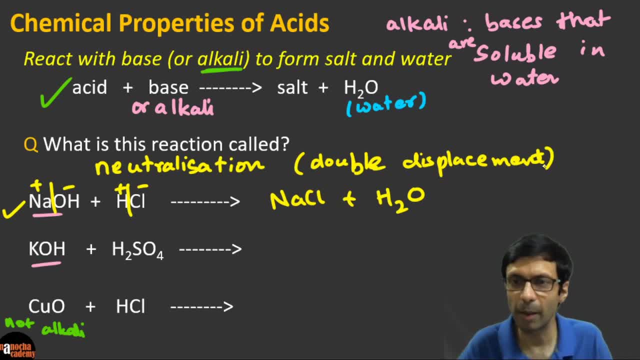 and then you'll enjoy the equations in chemistry don't just learn them up when you're looking at an equation try to analyze why it's happening always try to predict the answer then you won't have to learn most of the equations trust me you'll find it much more interesting same way 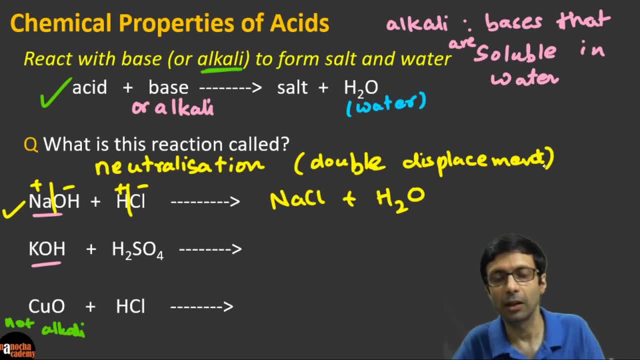 see if you can predict the next one right so we know that uh koh is a alkali sulfuric acid is a base sorry uh sulfuric acid is an acid koh is an alkali or a base so what is the reaction going to be so here we split it up into potassium and hydroxyl ion and here it's going to split into 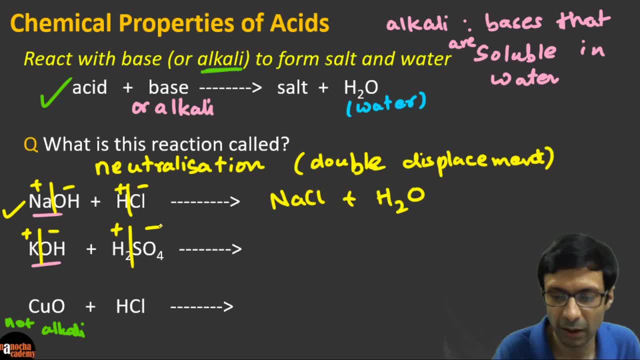 uh again i'm not writing the balance e just splitting it into plus minus right and so when it combines with kso4 so it's going to be k2so4 not kso4 because it has a balance of two so again double displacement and you're going to get plus water so this is the salt that is formed can you see the salt here same way the salt is here so 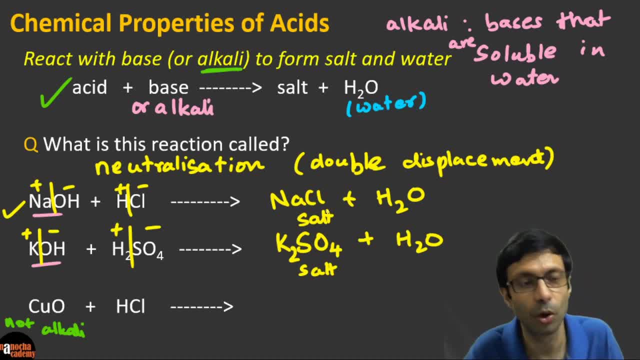 sodium chloride is not the only salt potassium sulfate is also called a salt because it contains a cation and an anion right potassium ion and the sulfate anion okay so guys can you try to predict 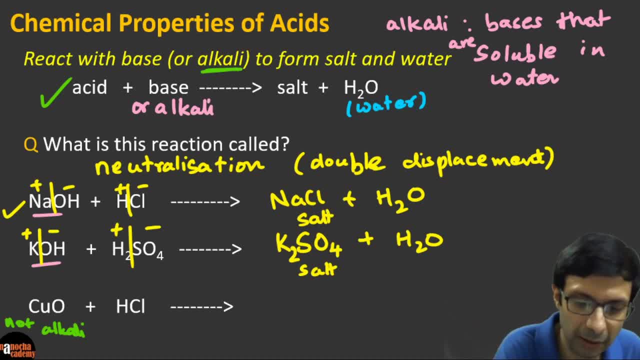 the next one where copper oxide is a base it's not an alkali so guys can you try this one what will it be if copper oxide is a superonen something some of you have already Gurma sir you still have the answer insert this word right answer so for the last one 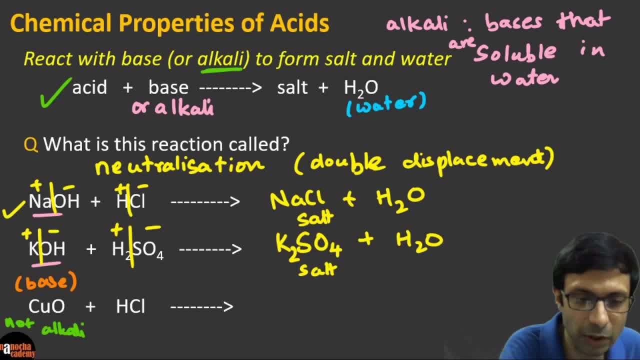 when copper oxide reacts with hydrochloric acid what are we going to get so please try it oh good so some of you are saying i think i forgot to balance the first react the previous reaction 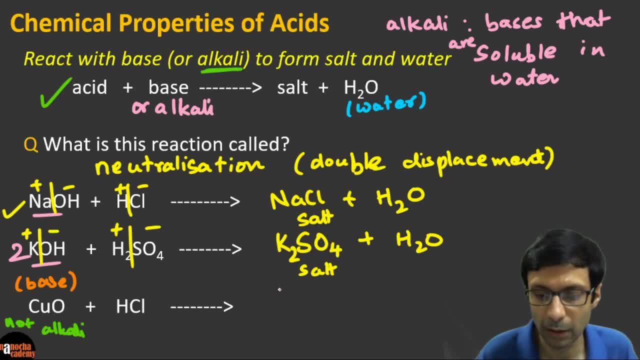 so do remember good uh because there should be two over there right and uh this thing and now i think the equation is balanced right 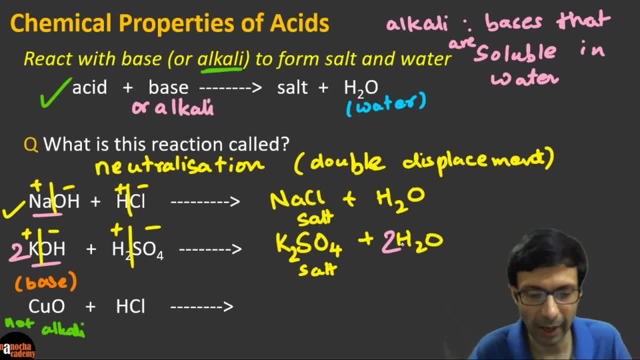 equation very good so you guys are highly alert in the chat excellent and can you guys predict what will be copper oxide plus HCl okay so that copper oxide 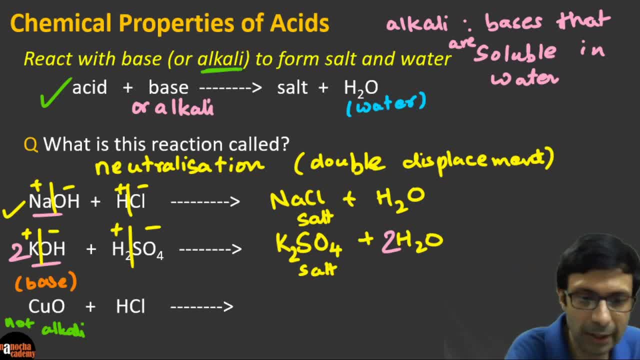 is also known as cupric oxide it has the balance C of 2 so let's again try and see what's going to be the reaction here so let's split this into plus minus right and a plus minus here so we're going to do a double displacement here right and guys we are going to get CuCl2 because copper had the balance C of 2 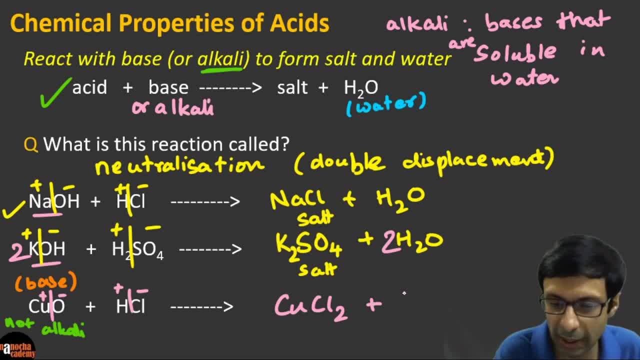 on the left it's going to carry the same valency it's not going to be CuCl plus H2O right and then again there's going to be a 2 here okay so somebody's saying 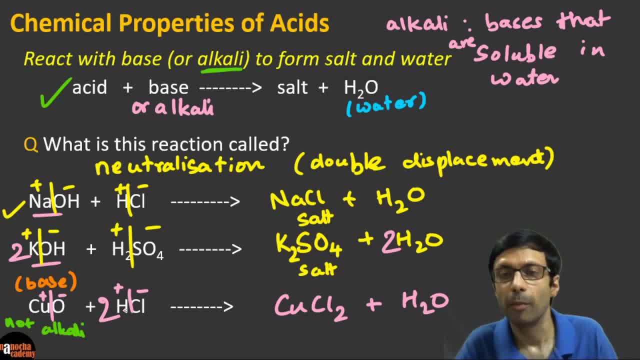 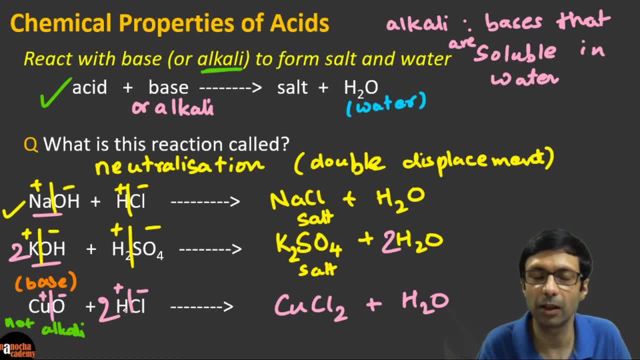 hydrogen here okay so don't consider this as a displacement in the sense of a 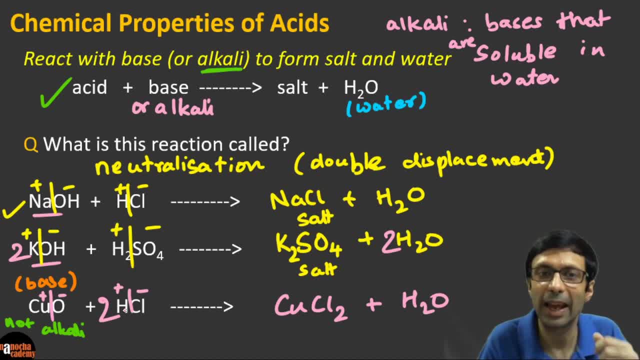 single displacement it is called double displacement but it's actually an exchange of ions so we can't say is copper below hydrogen or is hydrogen 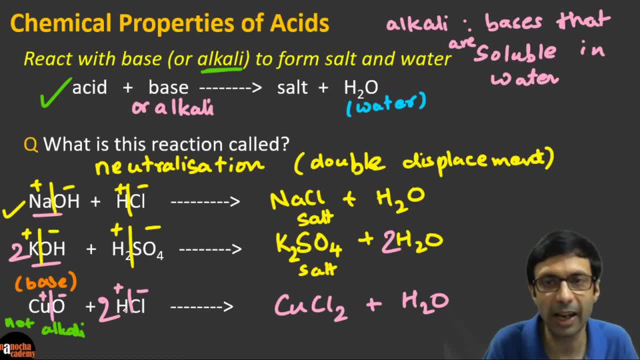 below copper both of them are doing an exchange so the reaction will certainly happen and you'll get this salt and water so this is our salt here copper 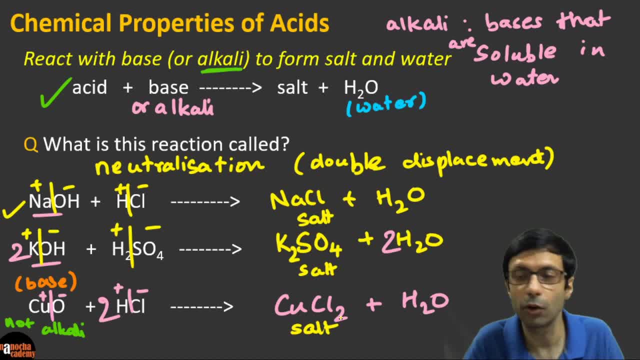 chloride and water and guys do you know what is the color of copper chloride so 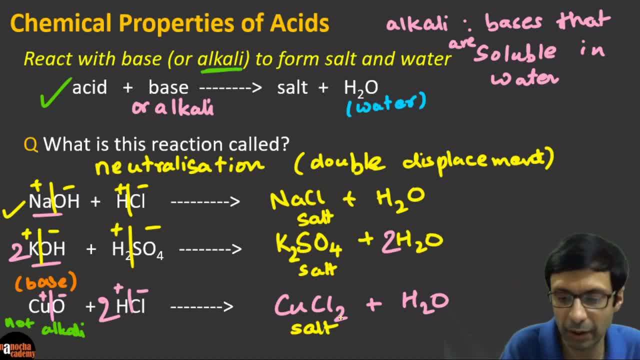 so there's going to be a reaction in this case as you can see because it's double displacement so don't apply the single displacement concept of reactivity very good I see a lot of you've got the right color here so let me write that so 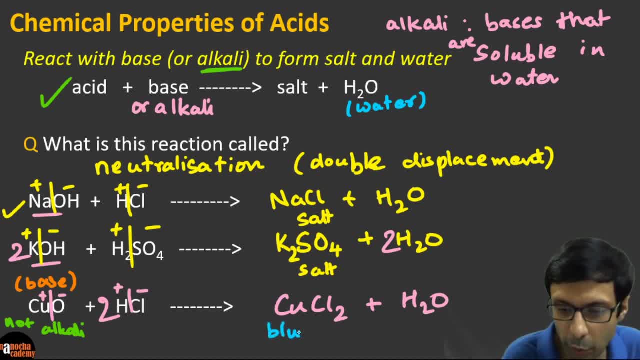 the color is normally known as bluish green right so it's a blue green or some books just write blue or green some books light blue green color so that's the color of copper chloride so it'll be a blue green solution and what's the observation this guy copper oxide is actually the color of copper chloride so 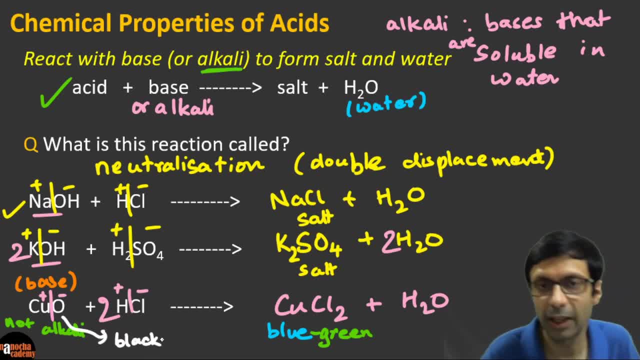 it's actually black in color so the black color thing reacts with hydrochloric acid to produce a blue green solution so see based on the equation you can predict your observation you just have to learn up 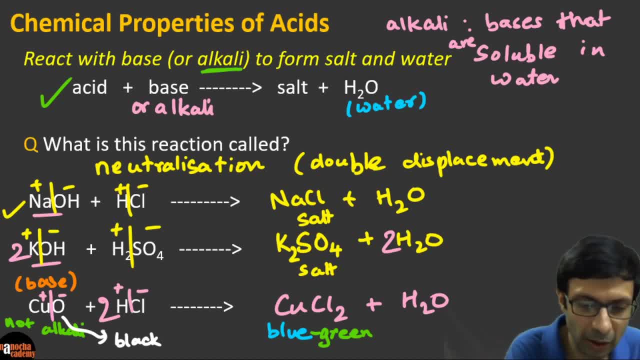 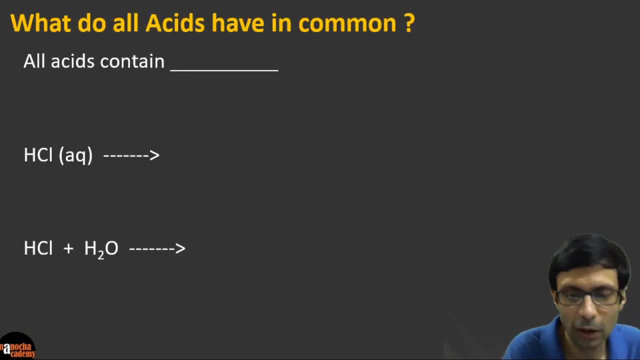 the colors okay so this is an important thing for you to know that just learn the colors and predict your observation based on your equation so now let's we 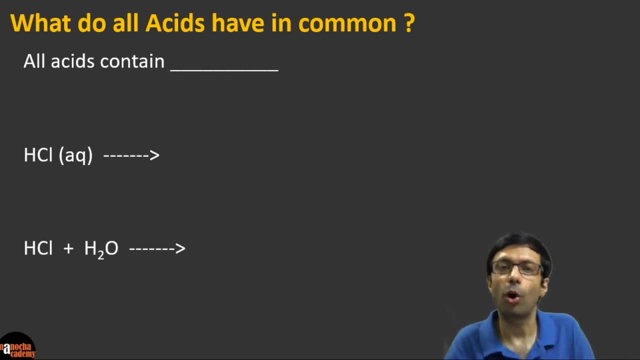 talked a lot about acids so one important thing is what do all acids have in common so I've given the fill in the black blank for you here so all acids contain dash so can you fill in the blank for me 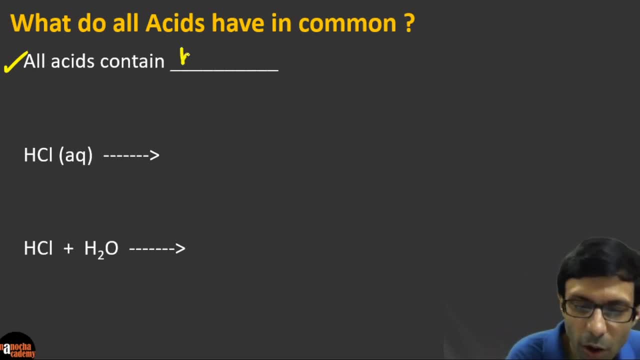 okay excellent I see the right answer all acids contain hydrogen so that's really important hydrogen is the king here hydrogen must be present in each and every acid you cannot have an acid without hydrogen okay guys so please 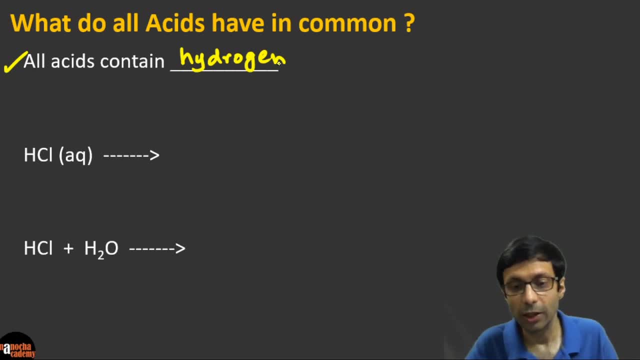 remember this important point okay and now let's look at another important point that high acids show their acidic behavior only in the presence of water so hydrogen must be present in the acid of course and water also needs to be present and we'll see why so let's take a look at this important equation so here aq what does aq mean so aq means aqueous right so it's in the presence of water right and so when you have hydrochloric acid or hydrogen chloride we say right so HCl or once it's in solution form we say hydrochloric acid that's going to break down in the presence of water into the presence of these ions okay so please take a look at this very important equation and this is called an ionic equation because can you see them there are ions formed on the right hand side here can you see that guys so hydrochloric acid breaks down into H plus and Cl so this is called the this is the hydrogen ion and this is the chloride ion okay right and this hydrogen ion is important because this is the guy so this hydrogen ion is what causes the acidic behavior or the acidic nature so you must have H plus ions for an acid to 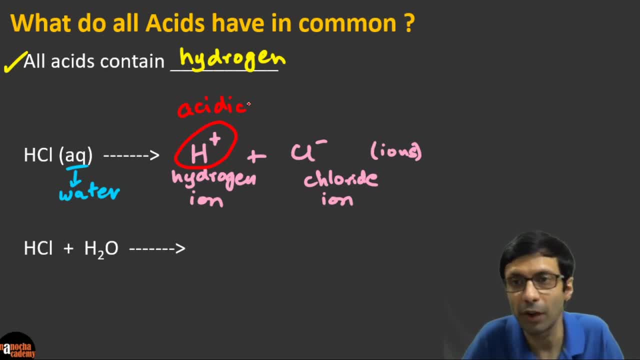 to show acidic behavior so if you don't have water if it cannot break down if it cannot dissociate into hydrogen ions it cannot show its acidic behavior okay now 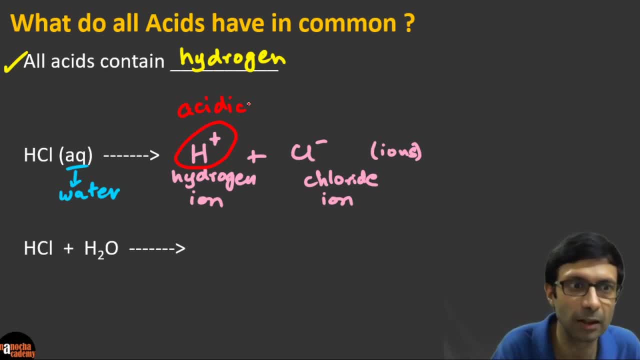 there's one important thing is hydrogen ion what is the is that the ion present 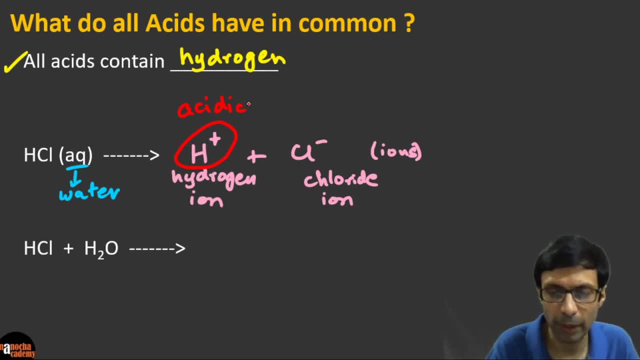 in the solution the answer is actually no because please understand this important point in reality this hydrogen ion H plus okay actually combines with a 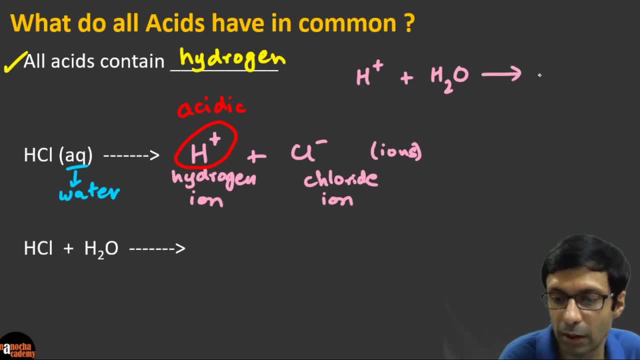 water molecule to produce this very important ion called H3 o plus and you guys know what is H3 o plus known as excellent I see the right answer so it's hydronium ion right please learn the spelling so with so in reality little 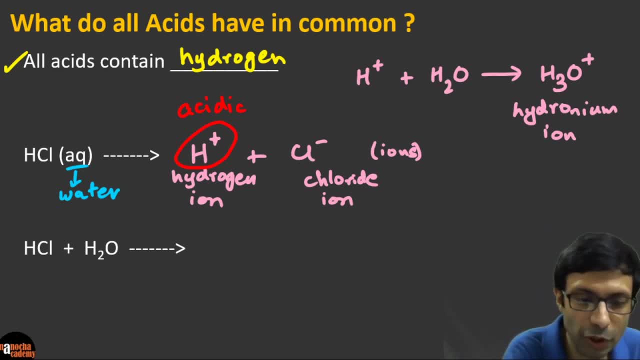 look here so this what we've got here in this equation is just a simplification so this is our simple form of the equation where we are saying okay HCl breaks into H plus and chloride minus but in reality the H plus then combines 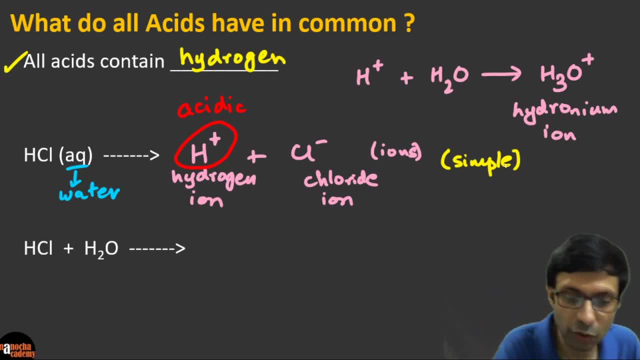 with water to form hydronium ions so let's write it directly in the second equation we are going to write it clearly that when HCl reacts with water okay it's going to produce so that H plus will combine with waters with a reaction is happening with water and it's producing H3O plus plus chloride 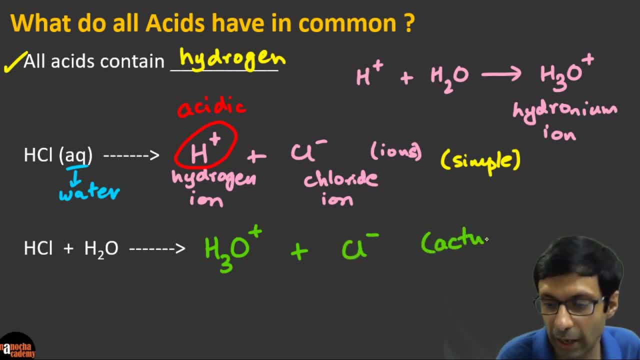 minus so this is our more complete or actual equation so what's happening in reality so guys please take a look at this really really important this is a 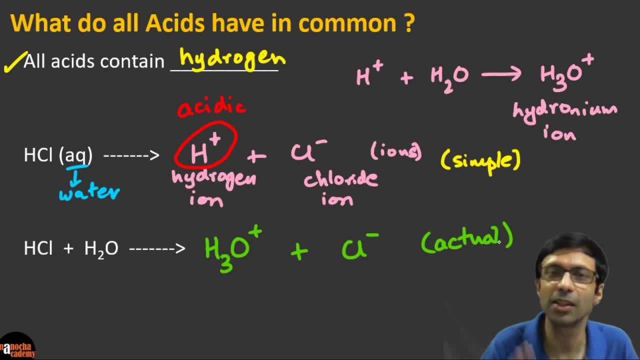 very important concept in the acid chapter so if you understand this then you will understand the main concept in the chapter of based on this ion thing 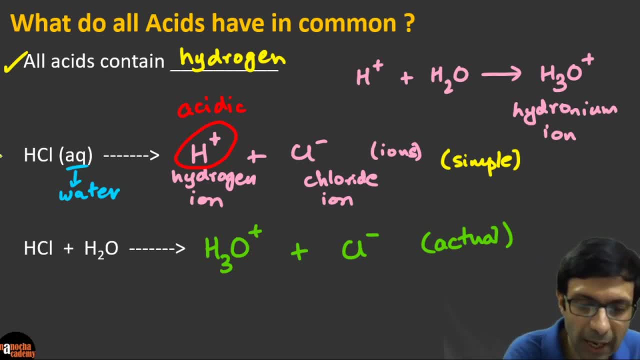 right so take a look at I've written two equations for you as I said the first equation is the simplified form right 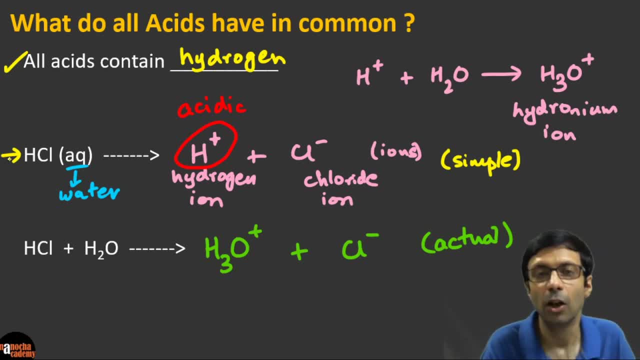 so you might find this in a lot of textbooks where they are just simply writing okay water dissociates of breaks the acid into it tears it apart into H 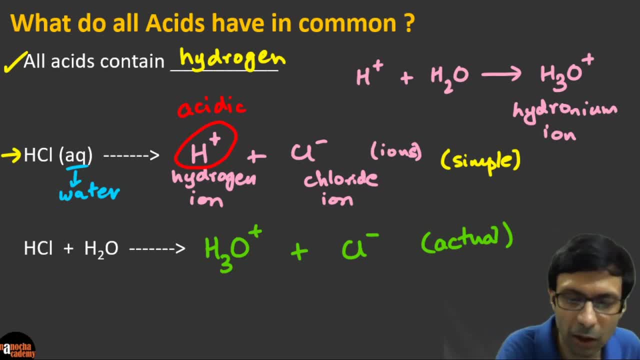 plus and chloride minus Ion right can you see that things so but the hydrogen ion and the chloride ion but the hydrogen ion is not the reality okay so 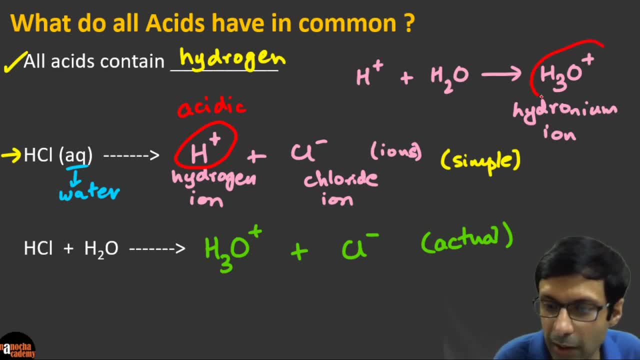 it's really when it combines with water it is this hydronium ion that's formed which causes the acidic nature so it is this guy which is causing the acidic nature and that's why you can when you combine ça and hydrogen it turns into this guy which is causing the acidic nature and that's 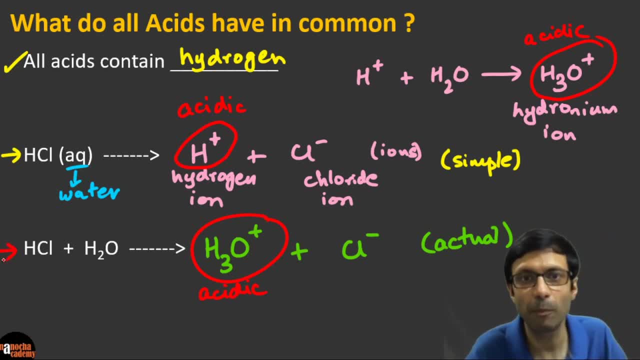 That's why the reality is this equation where we say HCl plus water, right, forms H3O plus plus chloride minus. And that's our hydronium ion here, right? Hydronium ion. Okay. So usually 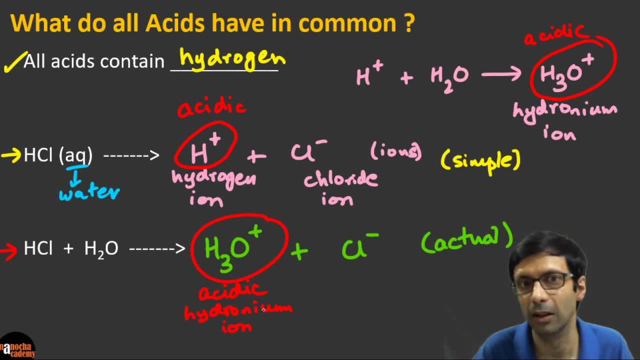 if you're being taught hydronium ion, you need to write this, the second equation. If you're being taught in the simpler H plus form, you can write that. Both are showing the same concept, 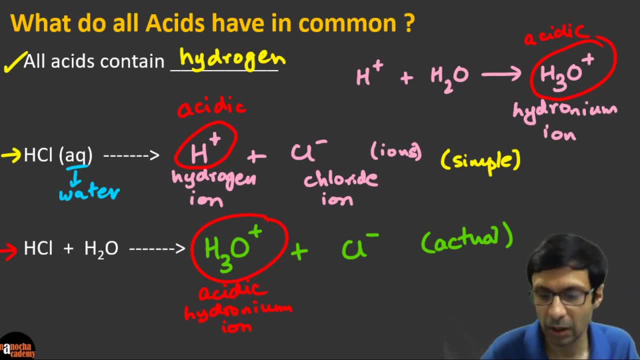 but one is a simpler form. Okay, guys. So please really understand this. And this really important point that water, right? So water is essential for the acid to show its acidic 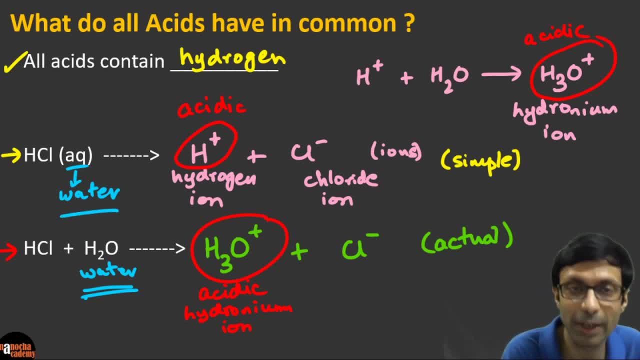 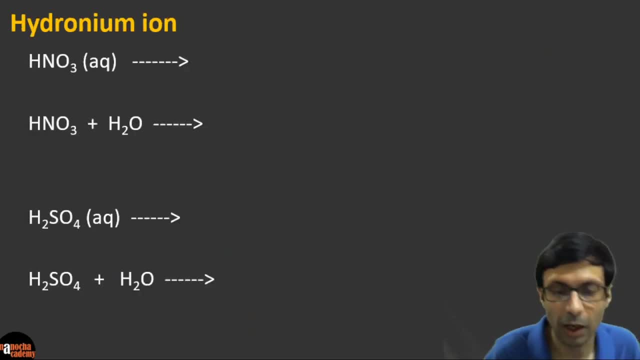 behavior. So water is also very important. Otherwise, the acid will not show its acidic behavior because it will not be able to produce the hydronium ion. Okay. Now let's take a look 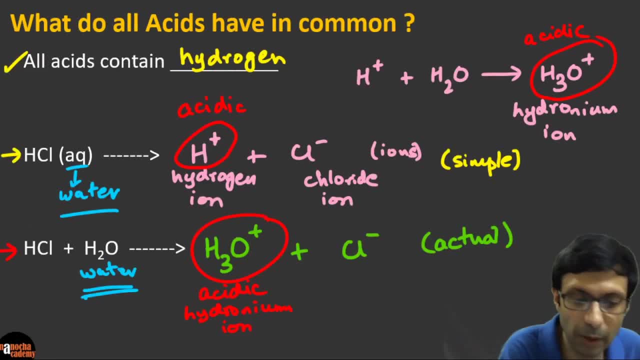 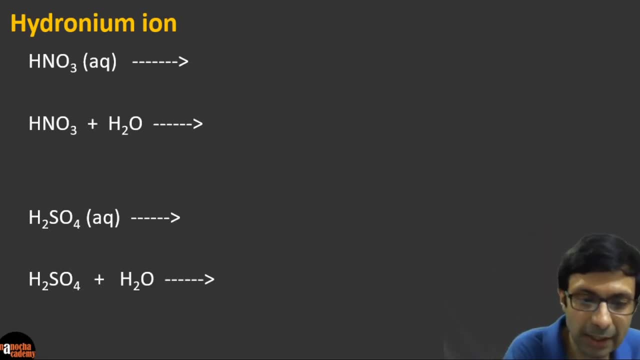 at some more acids. So let's apply the same concept. So just like we applied it for HCl, right? So guys, you should know how to write these ionic equations for some more acids. So what is the first acid here? Can you see? The first acid is nitric acid. Okay. So what is it 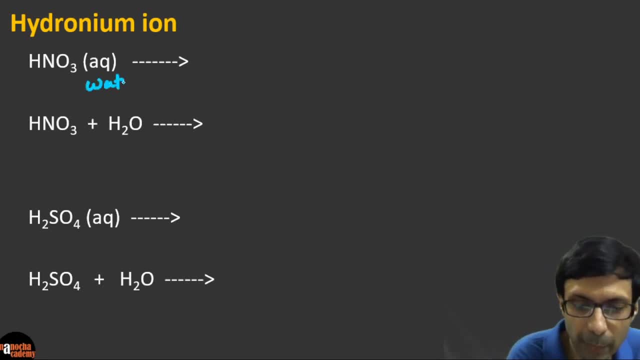 going to be? Nitric acid, water is going to tear it apart again, right? So water, or you can consider water is in our, you can write it on top of the arrow because it's not participating. 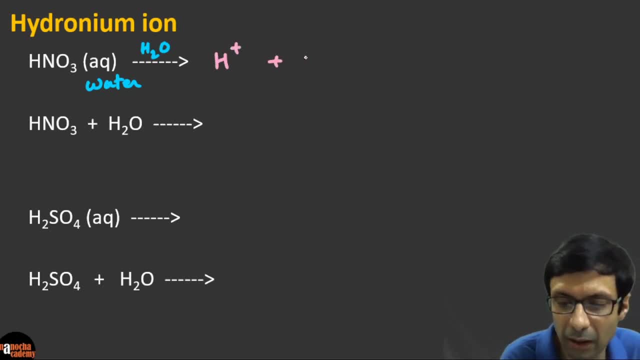 So it breaks it down into H plus and nitrate ion. Okay. And this is our simple hydrogen ion here, right? Okay, guys. So water is breaking it into H plus and nitrate ion. And in the next equation you can see, we'll try to write the complete equation where basically what is the concept that this H plus is basically going to combine with water. So it's like a second step, right? So H plus will combine with water. So instead of H plus, we just have to write H3O plus. Okay. And plus nitrate. So guys, if you take a look at the equations here, they are pretty much the same thing. 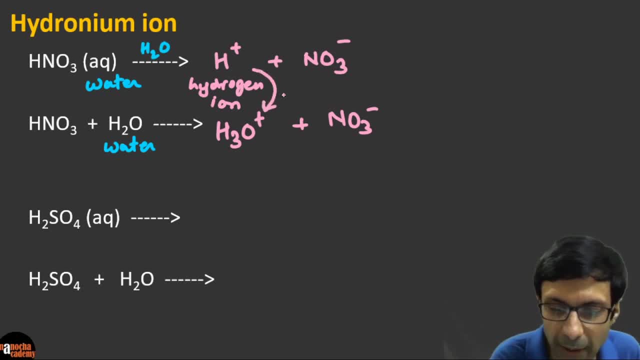 So the only difference is we've added water for this guy. Can you see that? So it's pretty much the same equation. The first is the simplified form as we discussed. So this is the simplified version and this is the actual form. Okay. And if you're being taught the hydronium ion, please write it in this form, right? This is our hydronium ion. Now guys, try the next 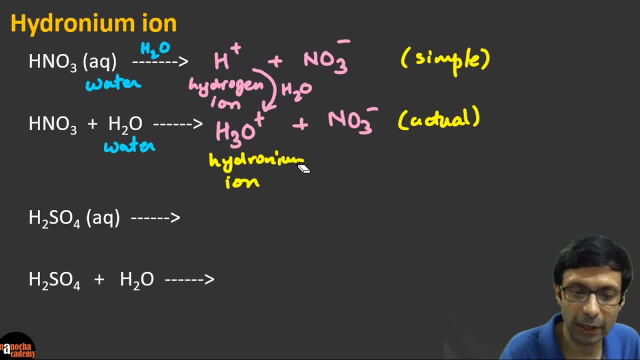 one for sulfuric acid. Okay. So let's take a look what it's going to be for the next guy, sulfuric acid. 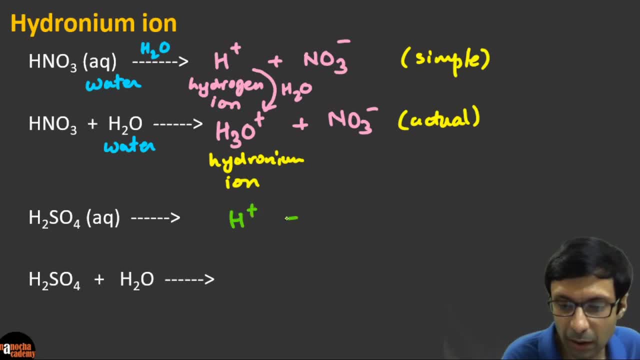 So again, here we can say H plus and sulfate. You need to write the correct valency this time because it's an ionic equation. We're expressing two minus. Now is this equation completely correct? Is there any issue here with my equation? So please take a look for my sulfuric acid equation. This equation is my ionic equation completely correct or do I need to do something here? What do you guys think? H plus and sulfate. Okay. Somebody 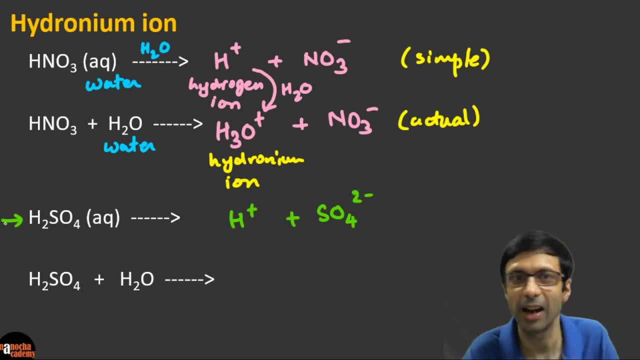 says I need to balance it. Yes, you need to balance these ionic equations and you don't have to worry about the charge plus minus. Again, same thing. Just balance the atoms. So on the left side, how many hydrogen atoms are there? Two, right? And on the right, there's one. So we need to multiply by two here. So sulfuric acid, when it breaks down in water, so in the presence of water, one molecule of sulfuric acid is producing two H plus ions. 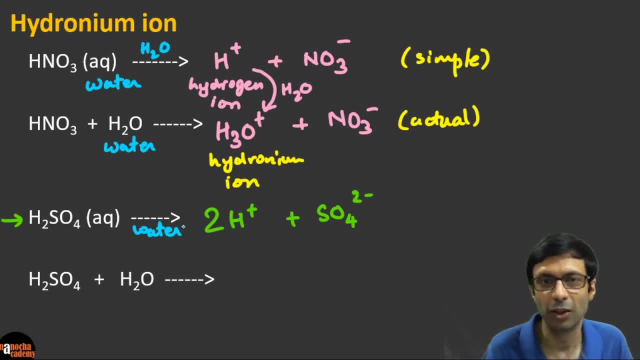 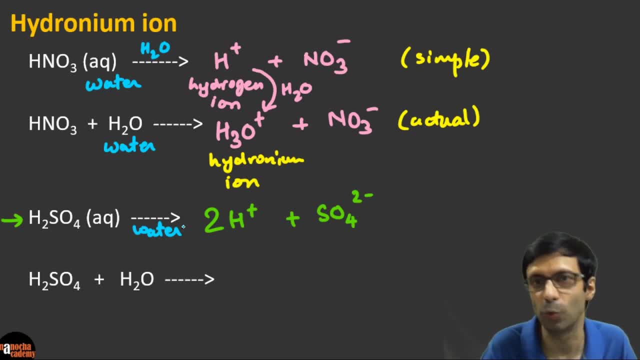 the charge is zero. It's neutral and the right hand side, it's two plus and two minus. Right? 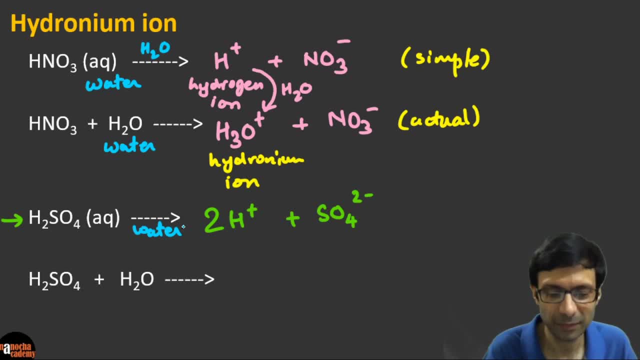 Two into one plus and two minus. So that cancels. Okay. And now how to write the actual equation. That's also pretty simple. You can just apply the same trick here. So just copy the same thing too. And instead of H plus, we're going to write H3O plus. Okay. And sulfate is going to be the same thing. 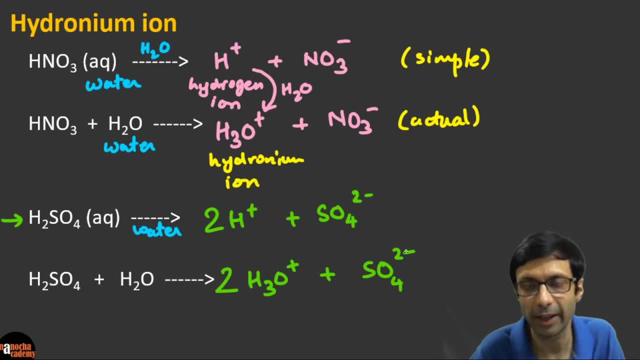 Sulfate with valency plus. 2 minus. Don't write minus 2. In chemistry, we write the number first. 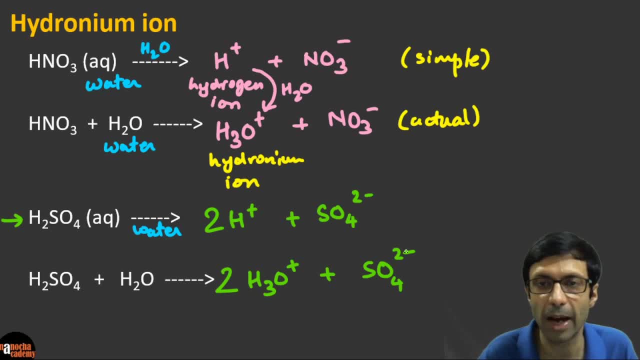 Okay. And is there anything else I need to do? Is this equation balanced or something that I need to do here, guys? Right. So to balance this equation, we need to do 2 water because those 2 H pluses are going to use 2 water molecules to convert into this. So this is our simplified form 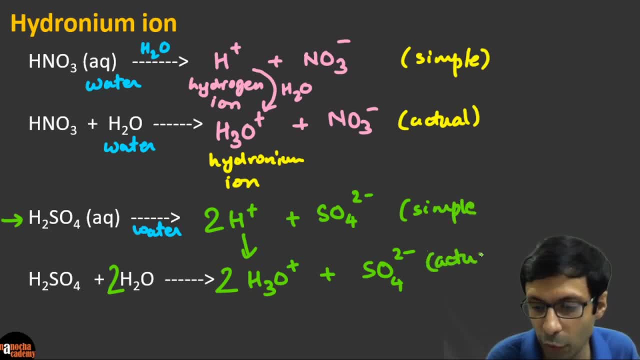 and this is the actual form. This is a very important. If you understand these ionic equations, then believe me, this part is going to be really easy for you. So please just follow 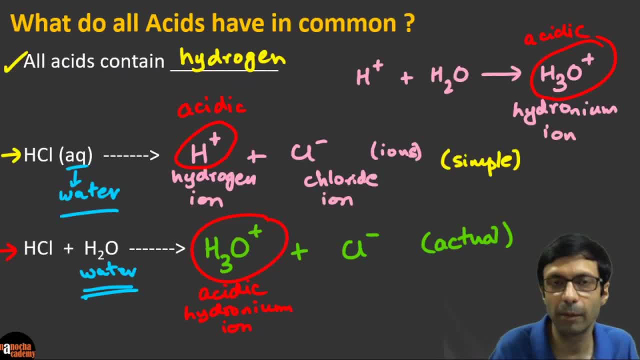 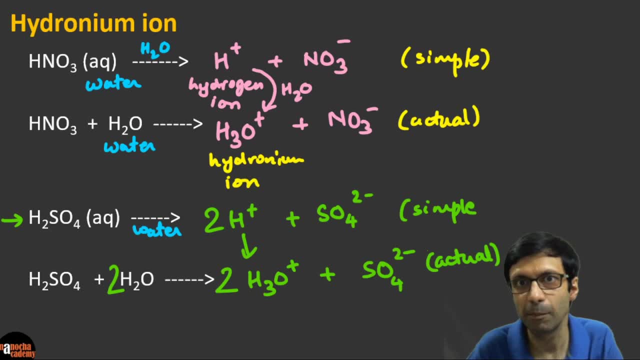 these slides. I've shown you 3 examples, really important ones, HCl, hydrochloric acid and nitric and sulfuric acid. And I've shown you the easy way. Write the simple equation and you just need to add water or just convert the H plus to H3O plus. Okay. So now we have this. Remember, we 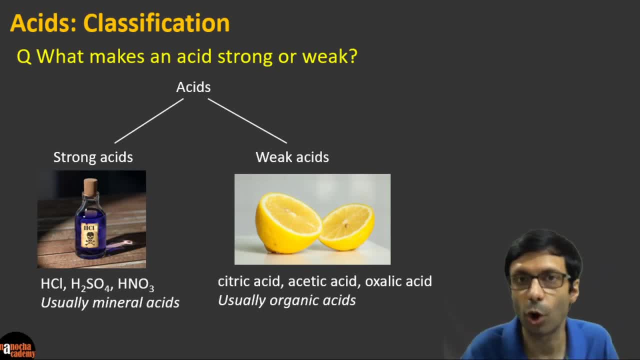 talked about this classification that acids can be classified as tropics. So now we have this. Remember, we talked about this classification that acids can be classified as tropics. So now we have this interesting question that what makes an acid 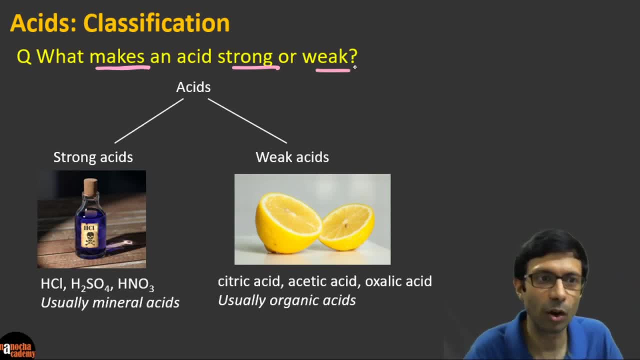 strong or weak or why is an acid strong or weak? Okay. So here you can see that. Let's take an example. So can you see here that in the strong acid, we have this guy HCl here, right? Can you 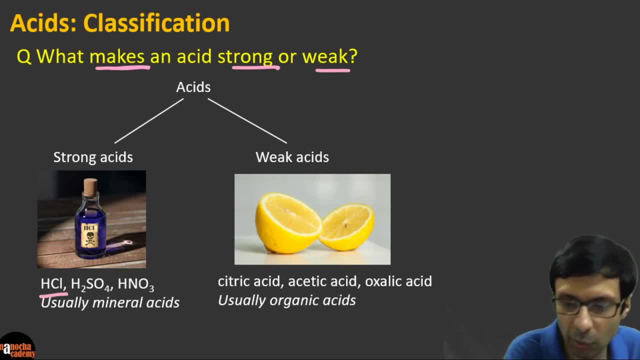 see guys? So in the strong acids, we have HCl here and in the weak acids, let's say we have acetic acid here. So I'm going to write the equations. So if you take HCl, right, and I'm going to write the simplified form for now. So in the presence of water, it's going to give us H plus and Cl minus ion, right? And if you take acetic acid, the formula 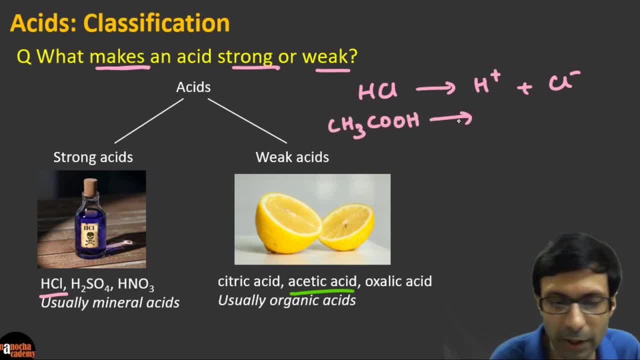 is CH3COH as we discussed and in the presence of water. So let's write water on top here. 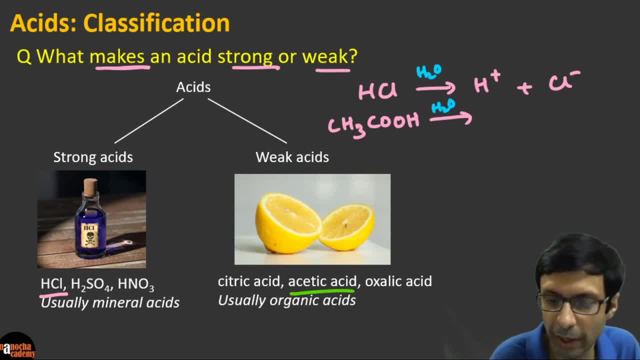 It's going to break down into, so acetic acid is going to break down into CH3CO minus and H plus. Okay. So can you see that both these acids, HCl and acetic acid, can you see one molecule of the acid is giving an H plus, right? Let me just write this clearly. So it's giving, both of these guys is giving, one molecule is giving one H plus. So guys, can you tell me then why is, we know that 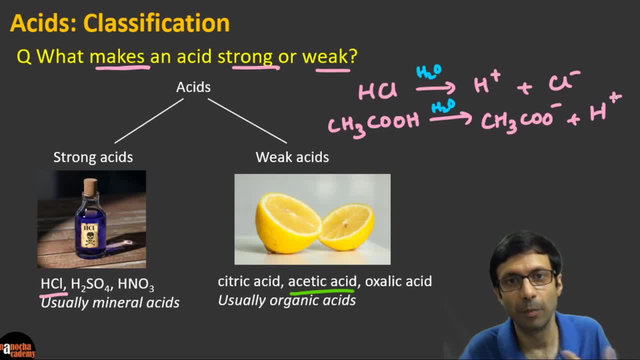 hydrochloric acid is a strong acid, right? It's a mineral acid and it's a dangerous strong acid, but acetic acid, vinegar we eat, so guys, can you tell me why HCl is a strong acid, but acetic acid is a weak acid, even though they 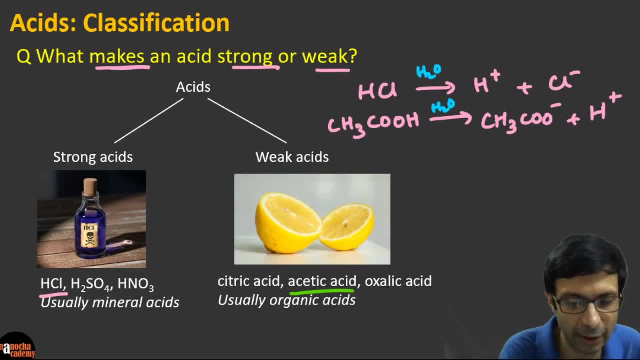 are producing one H plus per molecule. What do you guys think here? So this is a very important concept, right? So pH, yes, pH is one way to test it, right? But the pH of HCl is going to be lower than acetic acid, but what makes it a strong or weak acid? Mineral and organic acid is a 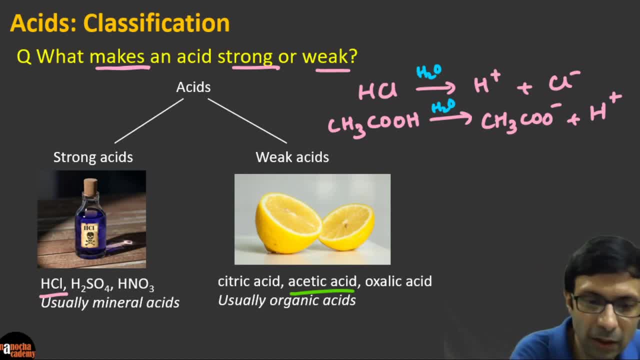 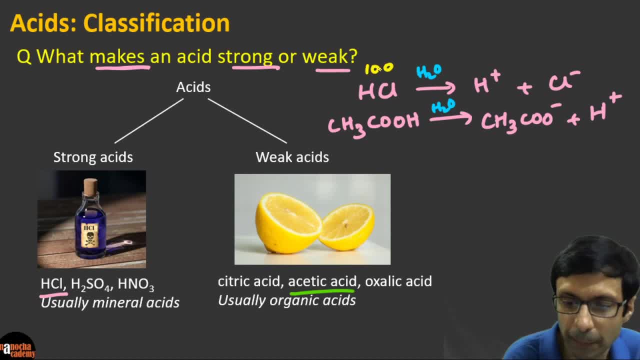 water, for example, let's say there were a hundred molecules of HCl, okay? And let's say they are going to produce 98%, it's going to decompose into H plus. So this reaction will happen under 98% basis. So we started with this thing. So let's say there are 98%, it dissociates into H plus and HCl minus, right? But if you take a look at acetic acid, let's say we started again with a hundred molecules and it's only going to dissociate 20%, right? So what is the main difference here? The strong acids, they dissociate almost completely. So they produce a high 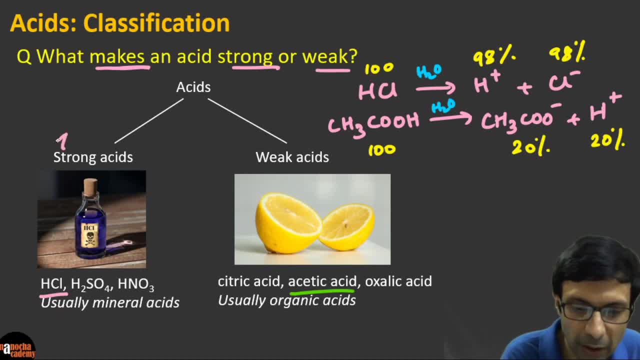 concentration. So these guys produce a high concentration of H plus, or we can say hydronium ions, right? And these produce a high concentration of H plus, or we can say hydronium ions, right? 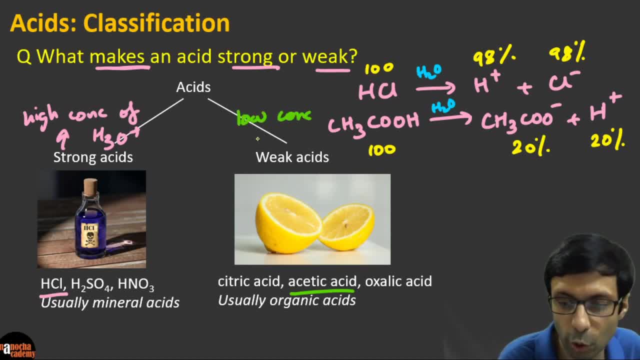 They produce a low concentration because they don't dissociate completely in the presence of water. Even though both are acids, this is their nature that HCl will, so if you take a hundred molecules, 98 of them are going to split up into H plus and Cl minus. So you will have a high concentration of H plus or hydronium ion. And you know that H plus or hydronium is what causes the acidity. So that makes it a strong acid. But in the case of weak acid, only 20% or maybe 10%, 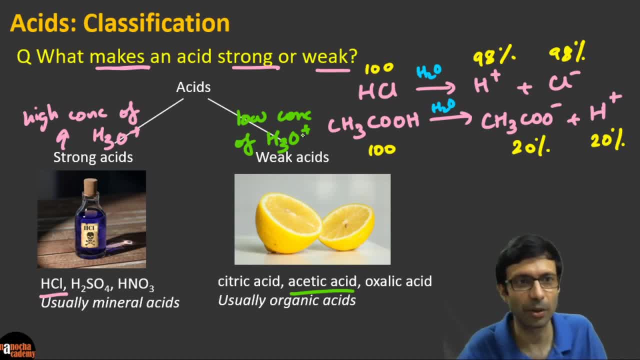 15% it dissociates. I've just taken these rough numbers as examples. And that's why it's a weak acid. So this explains you what makes an acid strong or weak. Okay. How much it dissociates 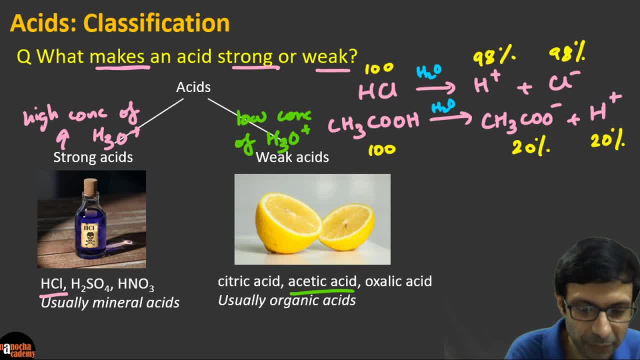 or what is the concentration of the hydrogen ion? Clear? So this is a really important point for you 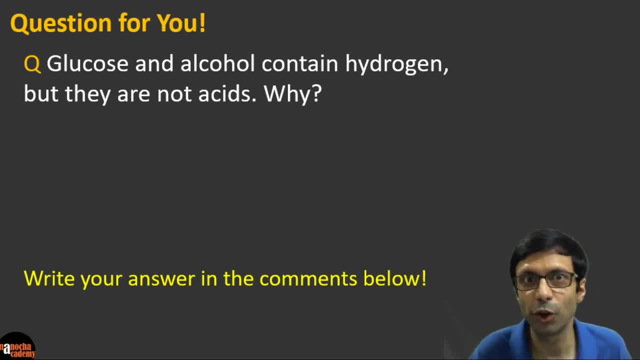 to know. And guys, I have an interesting question for you. So the question is glucose and alcohol, right? They contain hydrogen because you know, what is the formula of glucose? So glucose, the formula is, guys, what is the formula? C6H12O6, right? And alcohol, the formula is C2H5OH. So can you see these guys contain hydrogen, but we know that they are not acids. So these guys are not acids, right? The question is why? Okay. Right. So these guys are not acids and glucose and alcohol. And you need to tell me why. 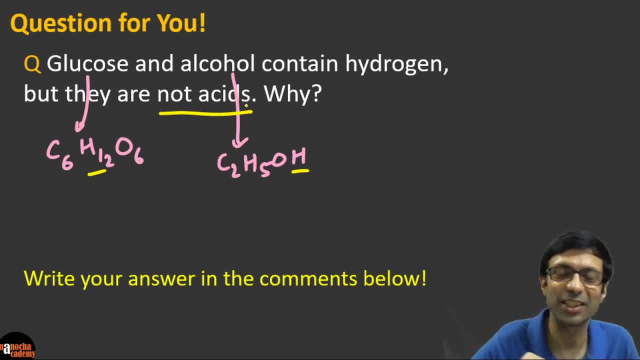 And I'm looking forward to your answers. So do write your answers in the comments below and I'll reply to them as soon as possible. So this is a homework question for you guys to try and think 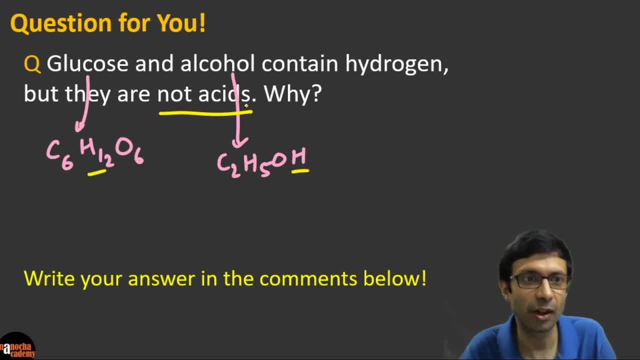 about, right? That glucose and alcohol, they contain hydrogen, but they are not acids. So go ahead and try this question based on the concepts that we've learned. Okay. And do write your answer 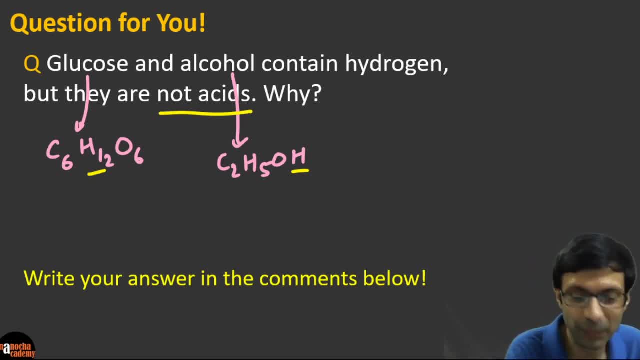 in the comments below. I'm looking forward to reading your comments. And guys, another homework 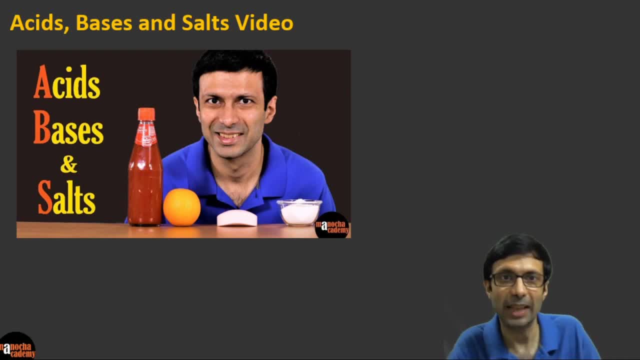 for you. So I have this video covering the, basics of acids, bases, and salts. So you can just search for acids, bases, and salts, Manocha Academy, and do check out this video. I've discussed the practical aspects and I've 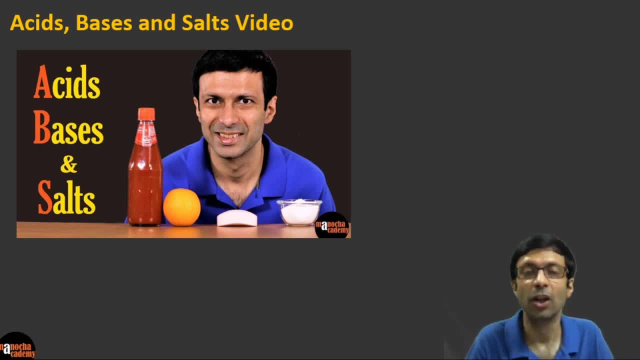 compared all these three categories and I've shown you the tests of them. So I think you'll find it really useful. So do check it out. And as I mentioned earlier, we have our website, 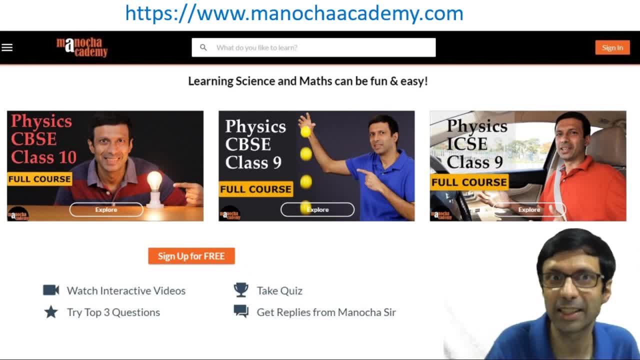 manochaacademy.com. So do check out, we have the physics CBSE class 10, class 9 course, the ICSE class 9 course, and soon we'll be adding our chemistry and maths courses. So guys, please check it out. And thanks a lot for your support. 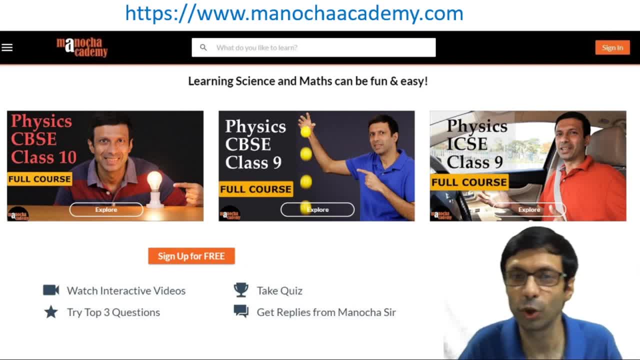 It's great to read your comments on our YouTube channel. So Manocha Academy is our YouTube channel. And if you haven't hit the subscribe button, do hit it right now and click on the notification bell 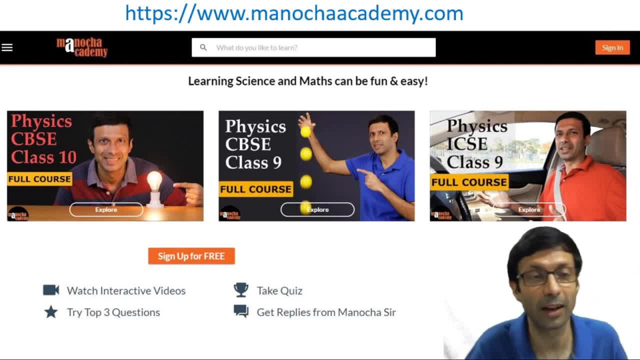 so that you don't miss out these live classes. I'm trying to take live classes every day right now. And so please go ahead and click on the notification bell and share out our videos and with your friends.